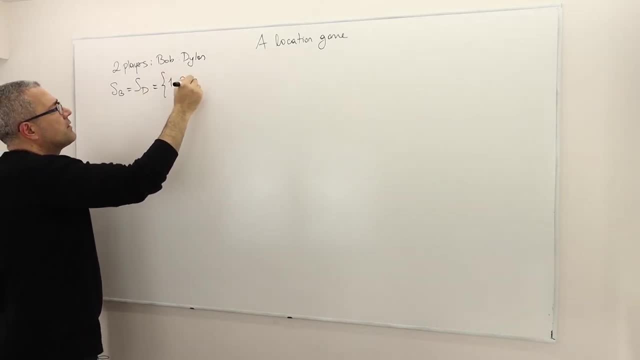 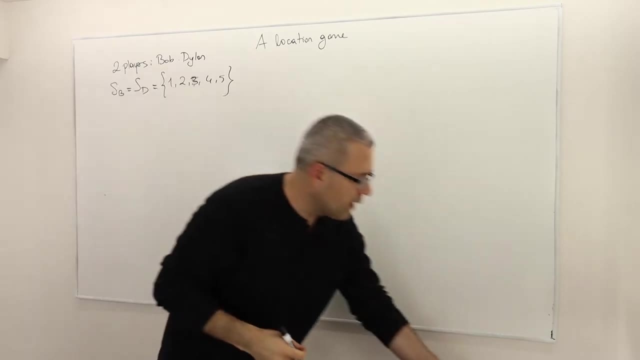 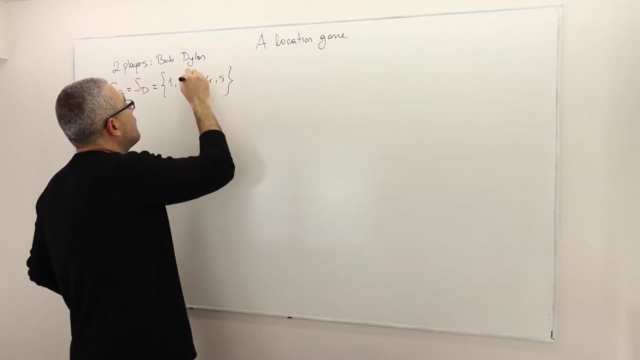 the Dylan's strategy set are the same And these are the strategies Oops: One, two, three, four and five. So, for example, strategy two means, you know, locating in a restaurant in sort of area three, And strategy four means locating restaurant at region four. So just to visualize, 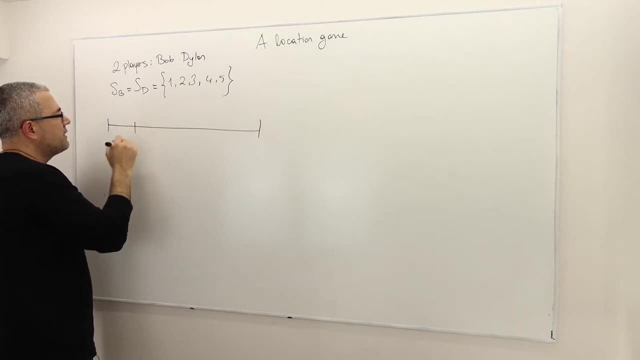 let's suppose this is the beach, and the beach is divided into five equal district or region. So region one, region two, three, four and five. Okay, So you may sort of misread the question and assume that the consumers who are going to buy pizza are also players in this game. 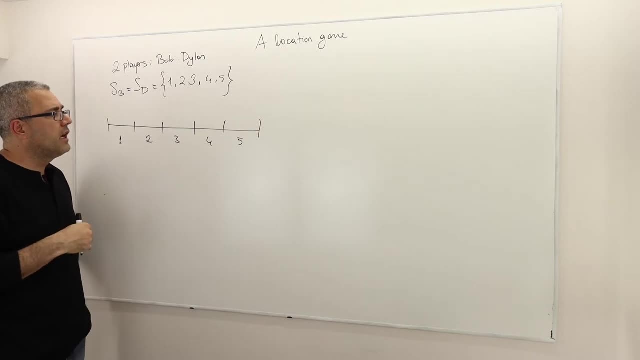 but they are actually not players in this game. Well, why is that? Well, if you read the question carefully, you'll see that the consumer's behavior is sort of given to you, And so that means we assume that the consumer's behavior 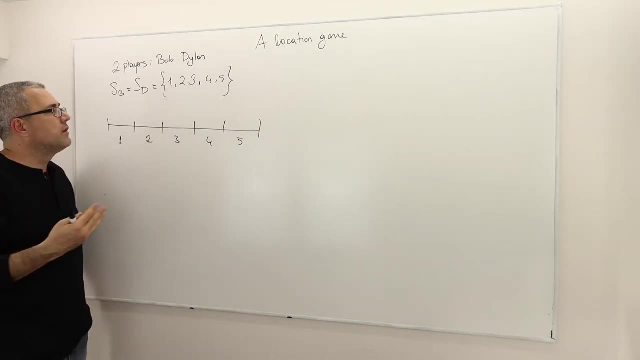 are fixed given. What is it? Well, the consumers always choose the restaurant that is closest to them, which makes sense, right? Because both restaurants are offering exactly the same meal- pizza- and both restaurants are offering at the same price. 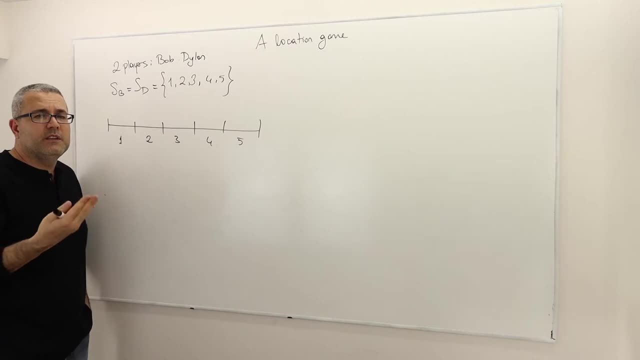 And so, ex ante, there is no difference between these two restaurants- Bob's versus Dylan- And so therefore, they choose. well, walking from one location to the other is, let's say, costly for them, And so they choose the restaurant that is closest to them. So it makes sense, But nevertheless. 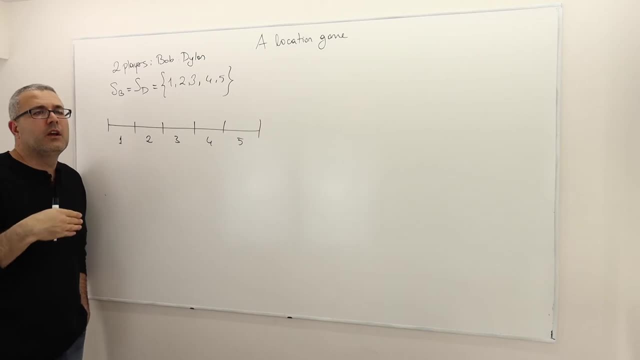 you can incorporate the consumers as a third sort of players, but that would complicate the game significantly, And so, just for simplification, we assume that there are only two players, Bob and Dylan, and these are their strategies, And the consumers basically just react to their choice location. 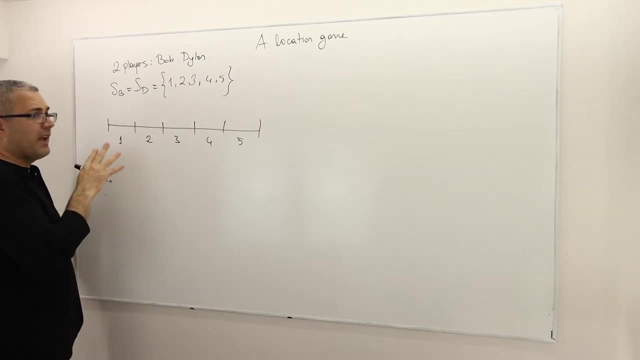 choice. So, as an example, if, for example, Bob opens his restaurant in region one and Dylan opens a restaurant in region four, for example, all right, so this is Dylan, this is Bob, And what happens is that all the consumers in region three, four and five will go to. 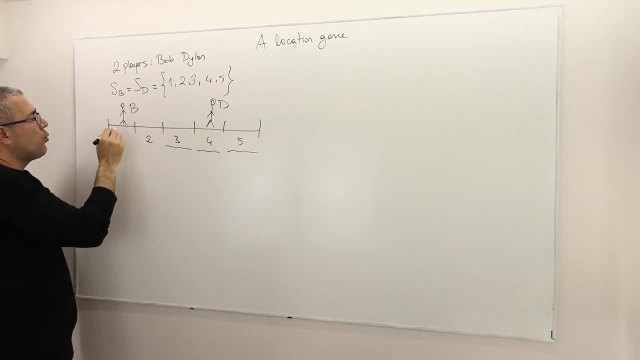 Dylan's restaurant and all the consumers in region one and two will go to Bob's restaurant, because the closest restaurant, for example, for a consumer in region two is Bob's restaurant and closest restaurant to a consumer in region three is the Dylan's restaurant. So these 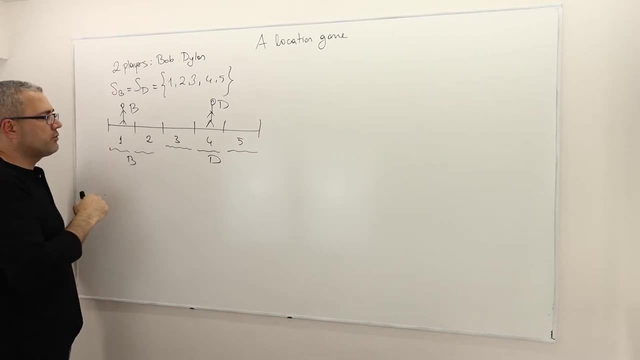 guys are going to Dylan's and these guys are going to the Bob's restaurant, All right, Well, obviously, sort of the not the scenario, but the outcome. well, that basically also determines how much you know net profits pay off each. you know Bob and Dylan will. 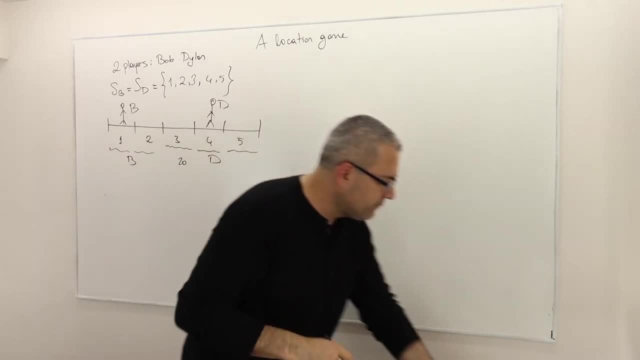 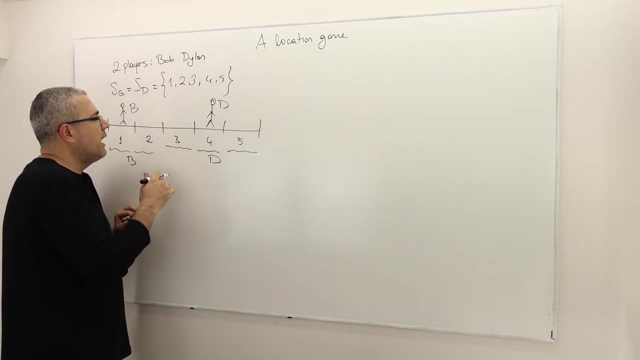 get. So 200,, I'm sorry, a thousand dollar. remember there are 50 customers and each customer spend $20 fixed, And so a thousand dollar if Bob or Dylan serves the entire 50 customers. So $1,000 from region three, $1,000 from regions four and the same from region five, which 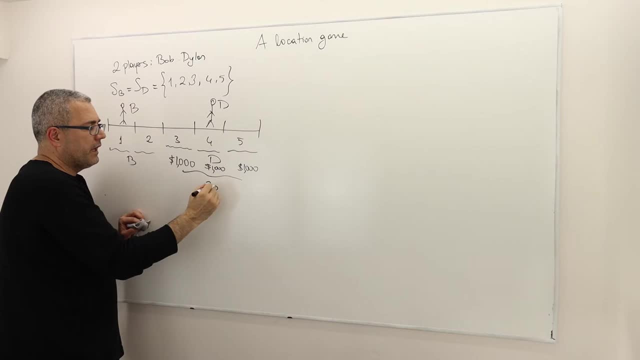 means the Dylan's payoff is going to be total of $3,000. All right, And the Bob's payoff is going to be thousand, another thousand, So it's a $2,000.. Oops for Bob. Well, the question is, can Bob, for example, increase this? Well, yes, of course. Uh, for example, 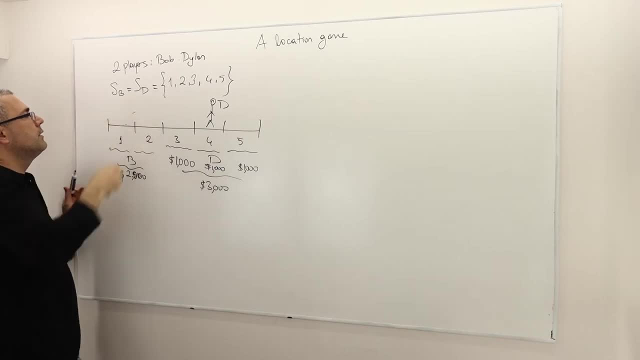 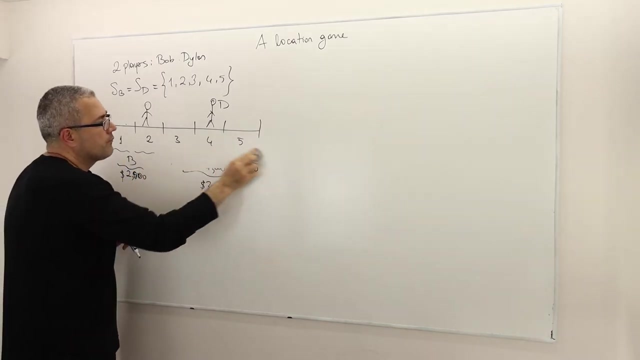 if Bob, Instead of opening up restaurant in region one, let's say he opens region two? Well, what about Dylan? Well, let's keep him in region four. What would be the scenario? Well, what would be the payoff distribution now? Well, this time, clearly, customers one and 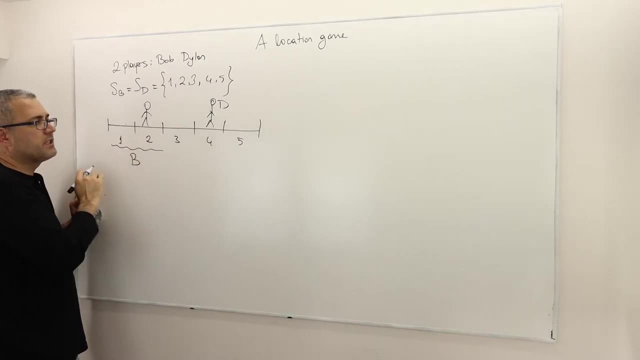 two are going to select a Bob's restaurant because it's closest to them, and same for four and five: they're going to go for Dylan's restaurant. What about the people in In region three? In region three, a customer will find both Bob's and Dylan's restaurants. 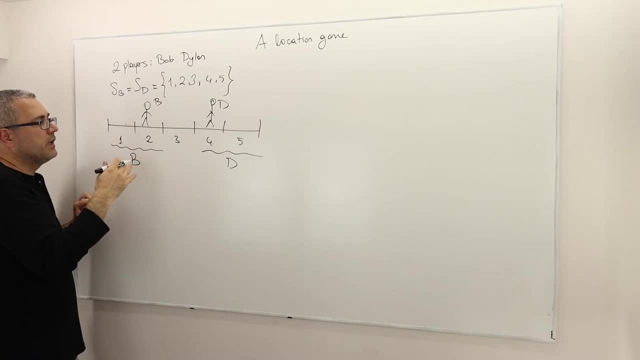 equal, so equally distant to his location. So therefore, the assumption there, if you again remember the question, because customers here are going to be split equally, So that means 25 of them will go to Bob's restaurant, 25 of them will go to Dylan's restaurant. 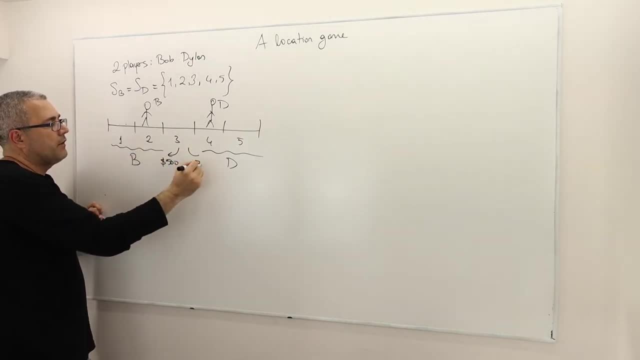 So that means $500 goes to Bob And $500 goes to Bob And $500 goes to Dylan. In that case the Dylan's net profit is going to be $1,000, $1,500, so $2,500. 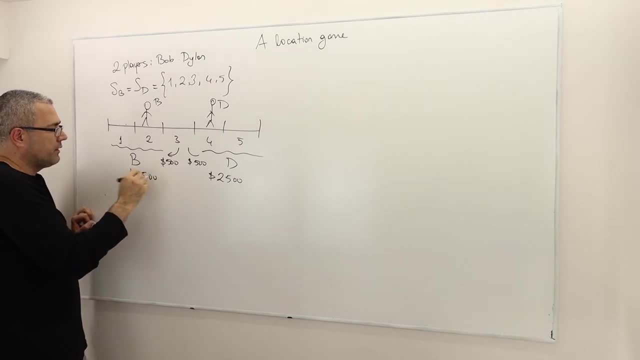 And same for Bob. It's going to be $2,500.. Okay, All right. So if you remember the previous scenario, the Bob profit was $2,000.. But now, by basically moving sort of closer to the Dylan's restaurant, he increased his payoff. 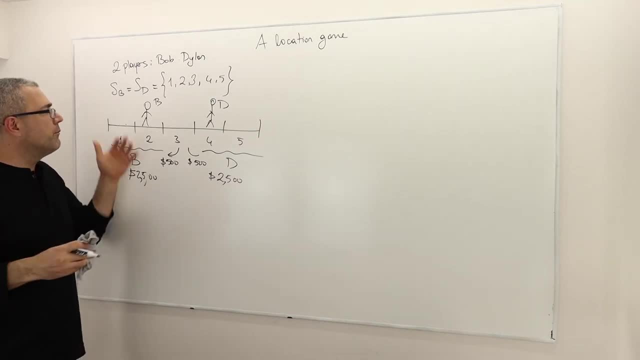 All right, But remember, so this is a simultaneous move game. Bob and Dylan decides where to locate his or her, his restaurant at the same time, simultaneously. And so the question was: what is the rational thing to do for Bob and Dylan? 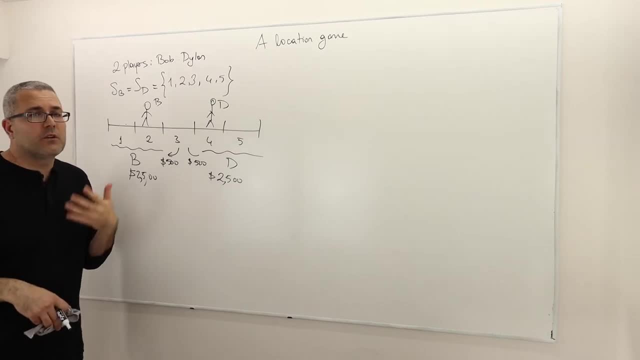 So which location is sort of the rational for these two fellows? All right, Okay. So what we're going to do? we are going to use the iterated elimination of strictly dominated strategies, And here is the argument. Let me first state the argument and then I'm going to prove this argument. 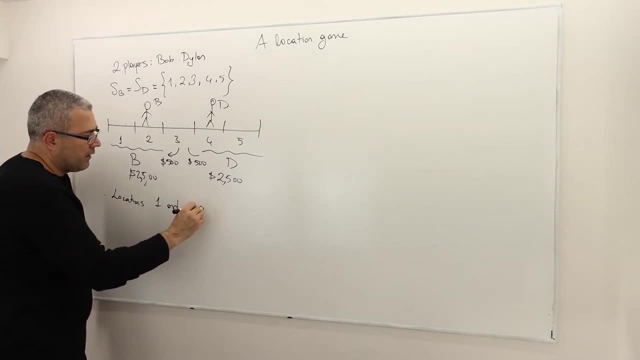 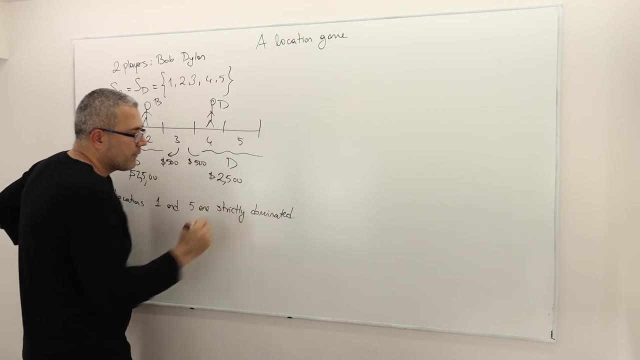 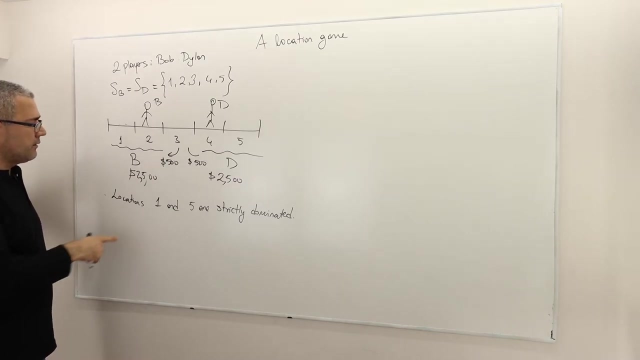 Locations 1 and 5 are strictly dominated by who? They're strictly dominated by, for example, locating. for example, location 1 is strictly dominated by locating in 2. And location locating in region 5 is strictly dominated by locating in region 4.. 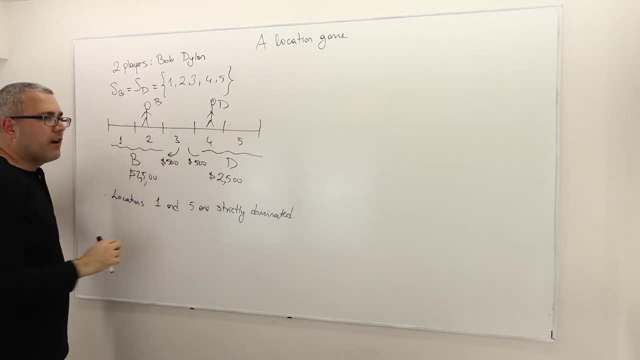 All right, But nevertheless, locating in 1 and locating in 5, sort of in the two opposite extreme, are strictly dominated. So that's going to be step 1.. And then step 2 of my argument. well, if locating 1- and oh, by the way, for who? 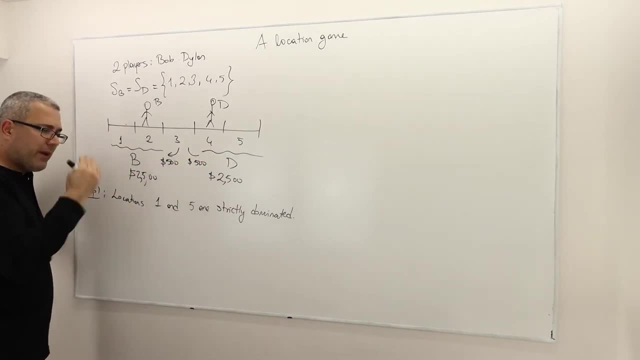 For Bob or for Dylan. Well, same For Bob and Dylan, for both of them, locating in either end is strictly dominating strategies And hence rational players. rational Bob and Dylan will never locate their restaurants in region 1 and in region 5.. 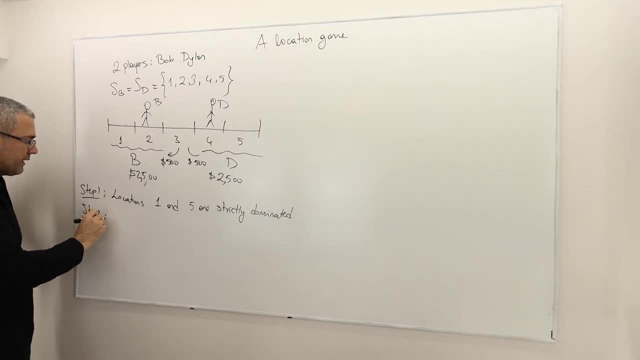 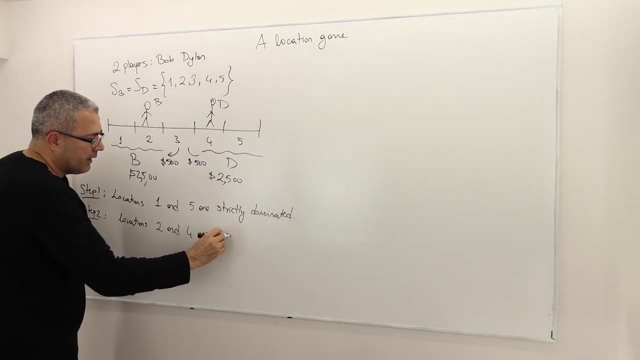 So, given this, I'm going to prove the second step. Locations 2 and 4 are strictly dominated. All right, So once 1 and 5 are out of picture, 2 and 4 are going to be the new extremes. 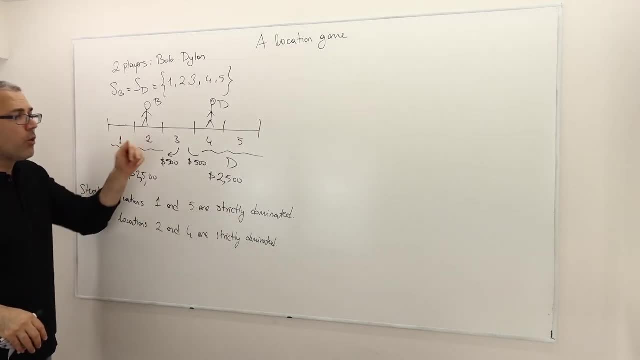 And what I will show that you know, locating in 2 or 4 is strictly dominated by locating in 3.. Okay, So then after this, the rational Bob and rational Dylan should also eliminate 2 and 4.. So that means there's going to be only one strategy available for each. 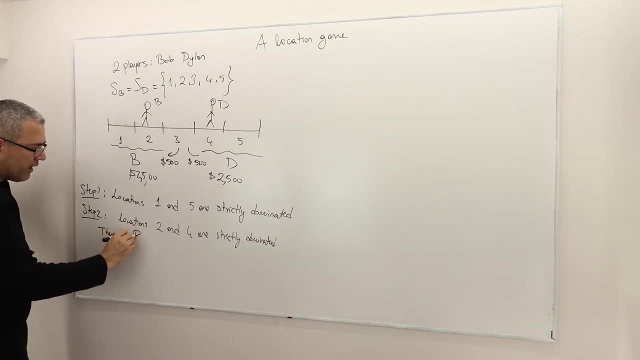 And hence, therefore, the rationalizable strategy for player 1, well, for player Bob and for player Dylan- is locating in region 3.. Okay, So that's going to be my conclusion. So, once again, the conclusion is that both rational players. 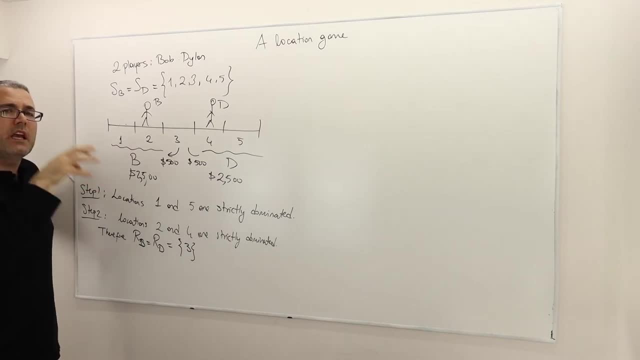 are actually going to locate their restaurants in the same spot, in region 3,, I mean, And that's the only rational thing to do in this game. And, by the way, to be honest, this conclusion has nothing to do. those payoff structure. 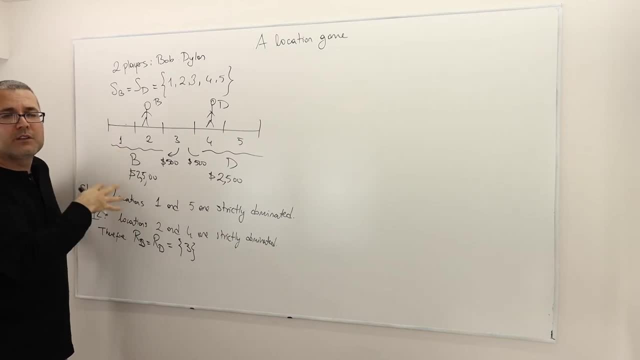 I mean whether it's $1,000 per region, $5,000, $1,000,000, it really doesn't make any difference. So that's sort of highly robust finding in this sort of environment. Okay, So let's prove this. 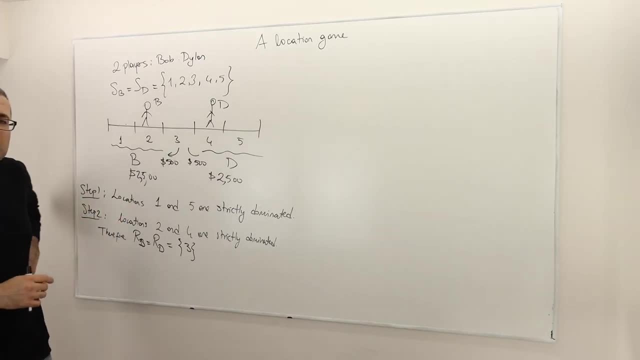 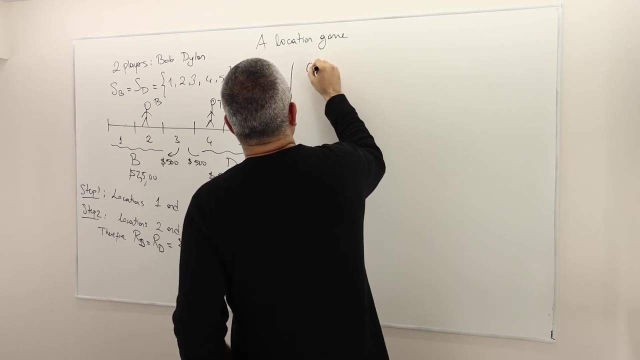 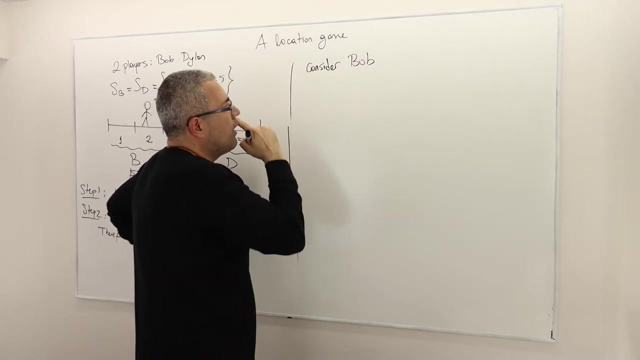 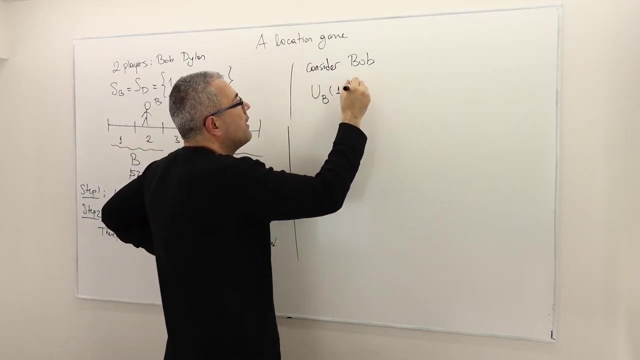 How do we prove step 1 and step 2?? So let's focus on step 1 first. If you want just fix one player, All right. So consider Bob, All right. Well, what is Bob's payoff if he locates his restaurant in region 1,, given that his opponent? 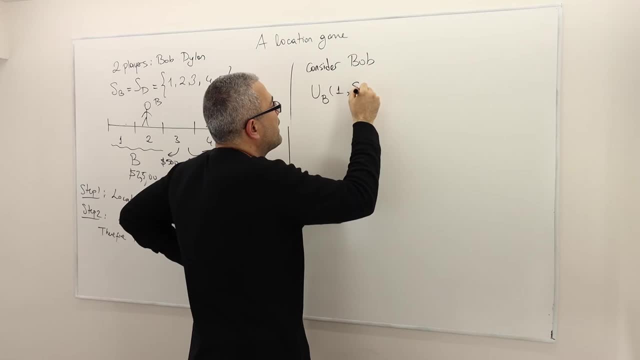 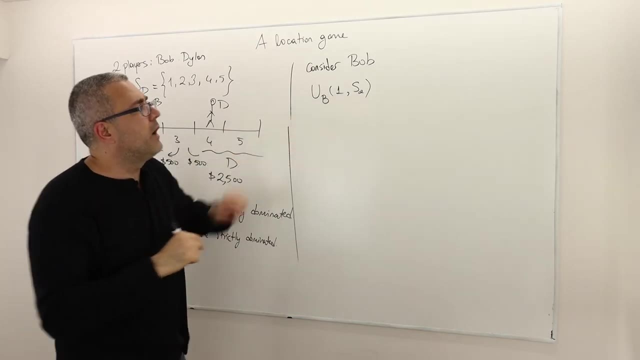 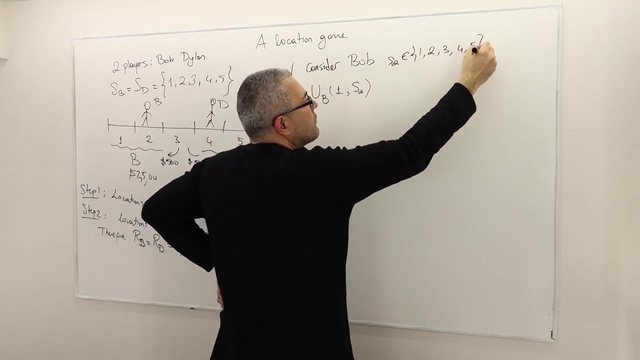 So I'm not going to denote it by significance. I'm going to denote it by S2.. His opponent, Dylan, is locating his restaurant in some region. S2 might be is a pure strategy, So it might be 1,, 2,, 3,, 4,, 5, right. 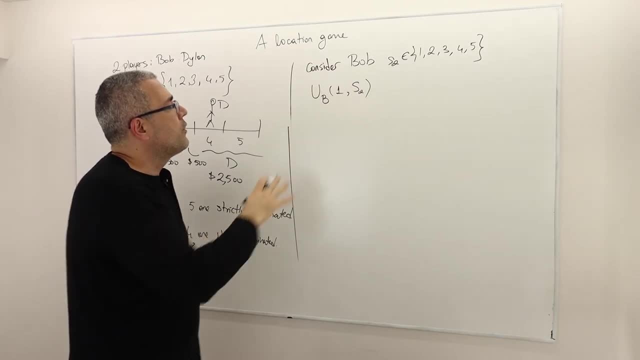 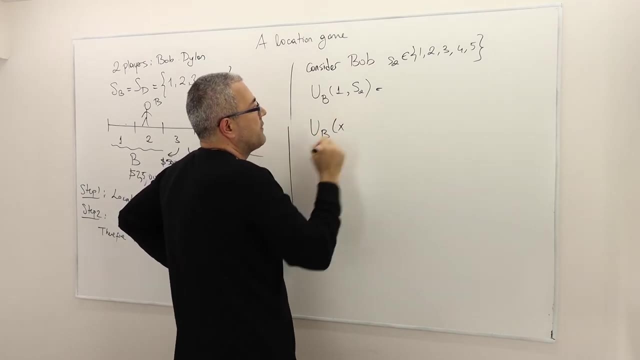 It can be any of those, All right. So what is this payoff? I don't know, But what I know is that is there any region- X All right- Where X is different than 1.. And obviously X is either 2,, 3,, 4, or 5, such that UBXS2 greater than strictly greater. 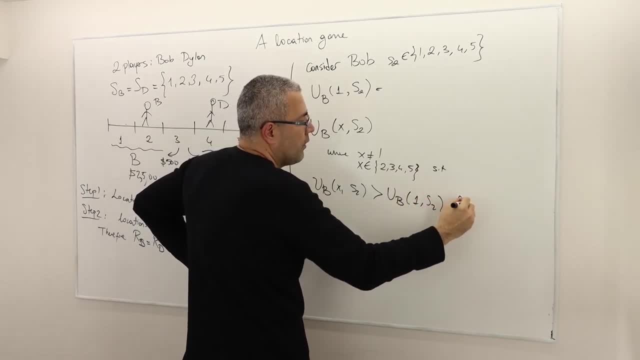 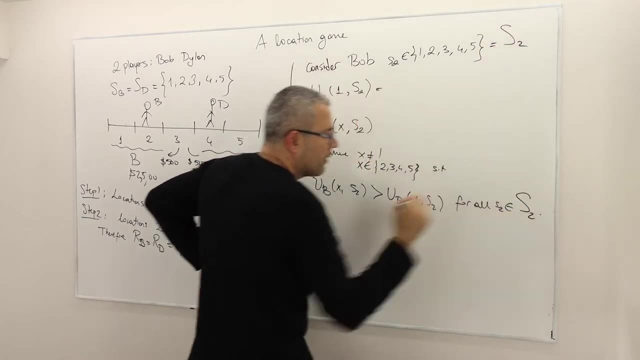 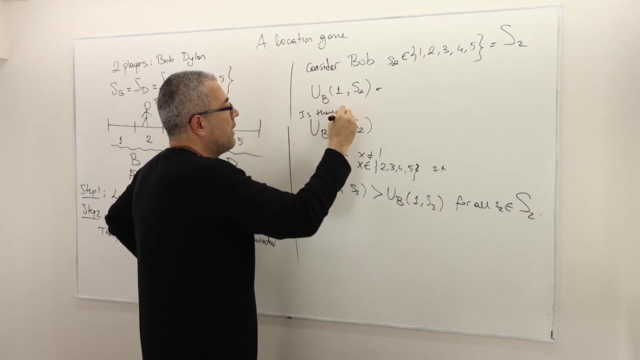 than UB1S2 for all S2 in this set. Let's call this S2, capital S2.. All right, So is there any? All right, Is there any? Is there Is there any X? So maybe I should put this: is there any X here? 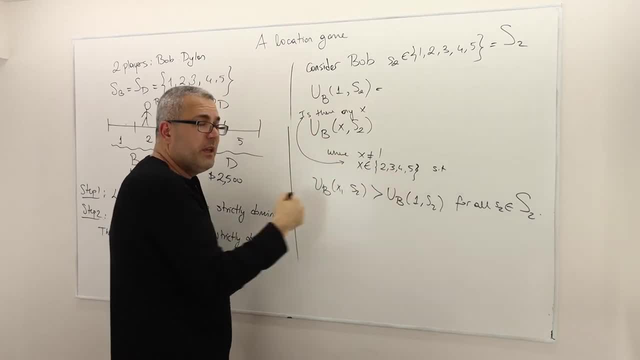 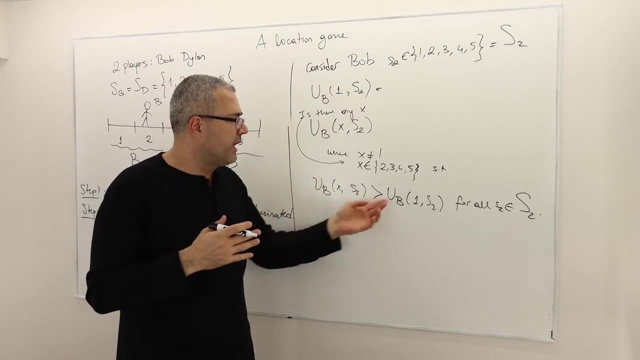 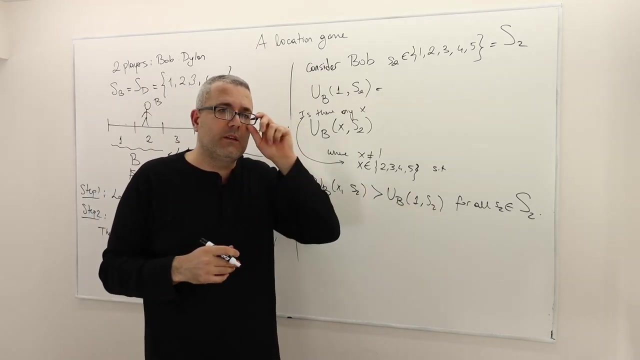 Is there any X which is an element of 2,, 3,, 4, or 5, meaning different than 1, such that the payoff of playing this strategy is always better than payoff of playing strategy? 1. Always means, for you know, regardless of what the second player, Dylan, does. 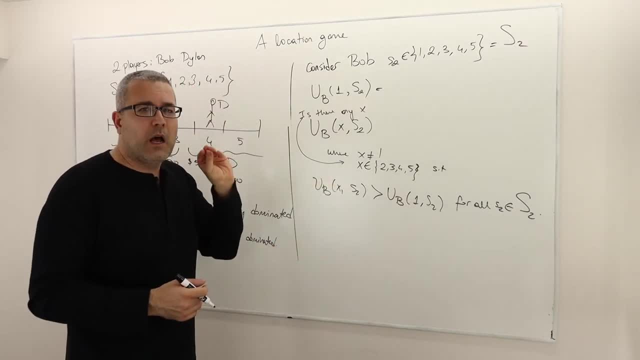 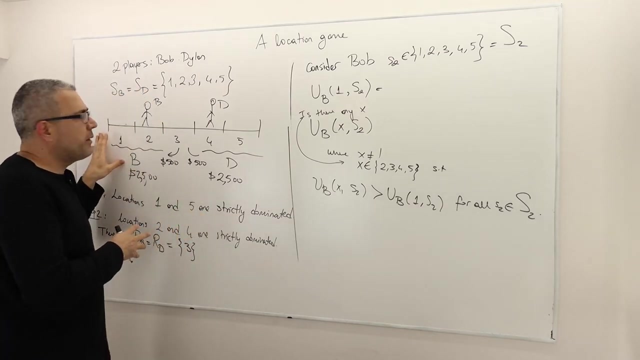 All right, All right, So this is exactly All right. So this is exactly what I'm searching for. Is there such X? If there is, well, then that means playing 1 is a dominated strategy. All right, With a very similar argument, because you know, there's nothing special about 1.. 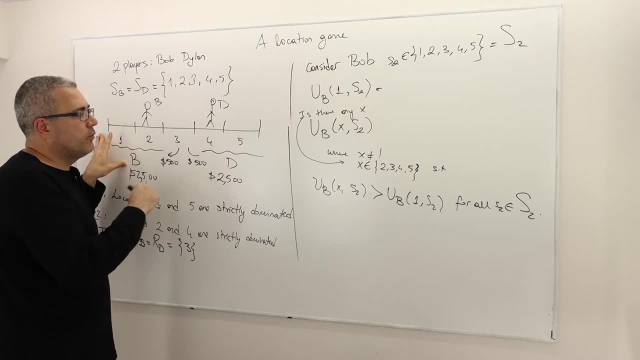 It's just an extreme point, With sort of a symmetric argument. I mean, if I can find X, I will probably do. I mean make the same arguments for 5.. Just take the mirror image, All right. So for example here: if X, 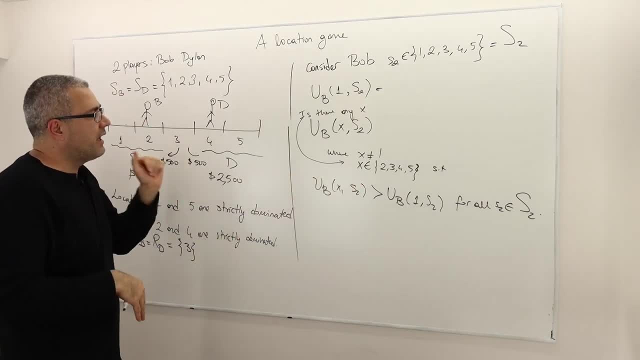 If X is equal to 2,, for instance, I can say that here, when you know selecting 5, is selecting 5 rational strategy or not. when I want to answer this question in this case, I'm going to show that X is equal to 4.. 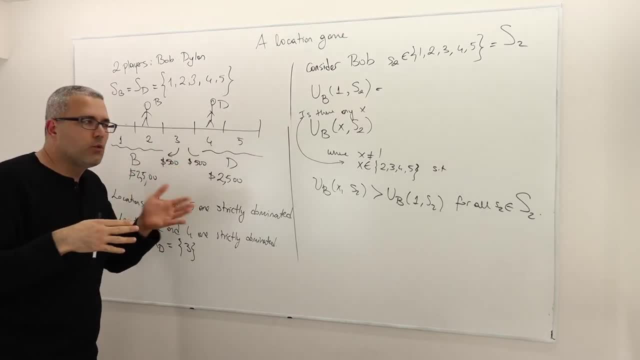 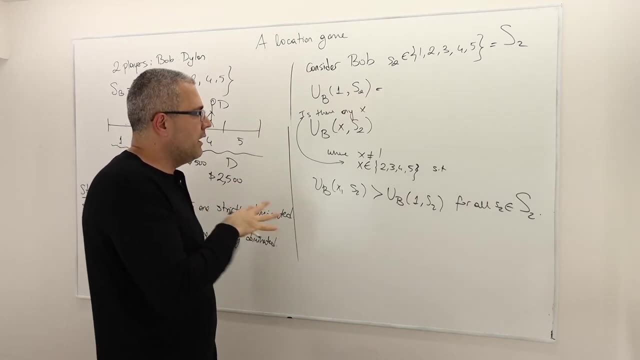 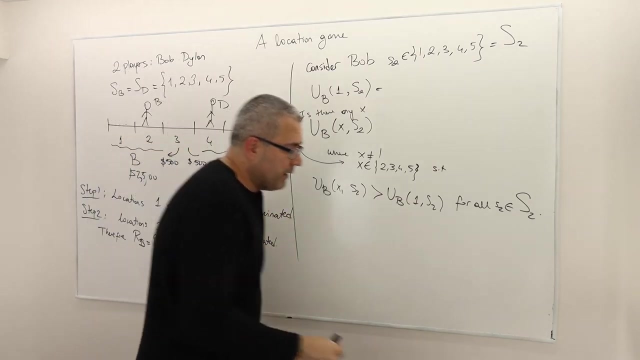 So it's a symmetric argument and so we are going to ignore repeating ourselves, But for the sake of completeness, I am going to do either way, Both ways, I'm sorry, All right. So let's see. I mean, what I need is, obviously, I need to understand what Bob's payoff will be if 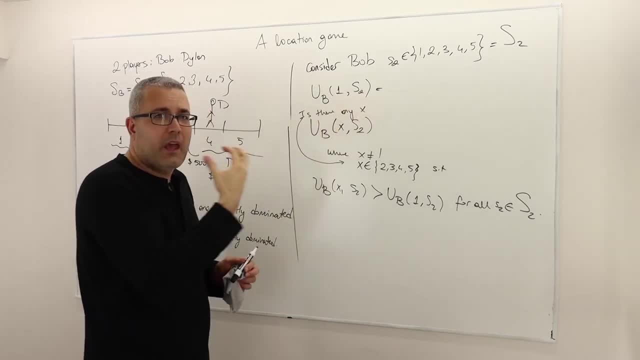 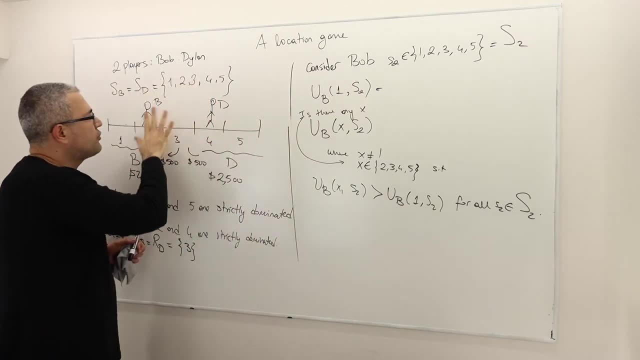 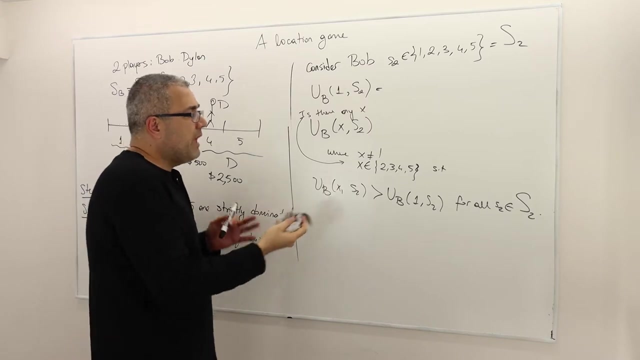 he plays 1,, but obviously the payoff will depend on S2, right? And so when you change S2, the consumer's distribution between Bob and Dylan will also change and hence the payoffs will change. So therefore, maybe the best thing. 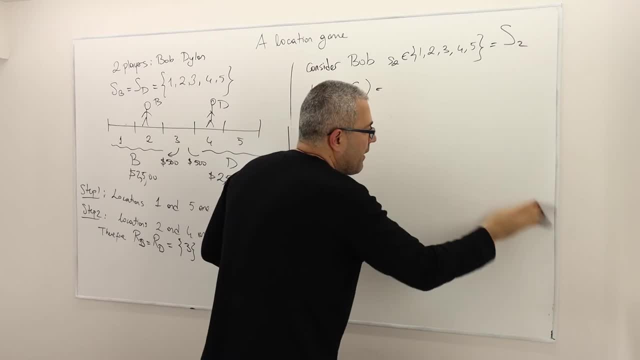 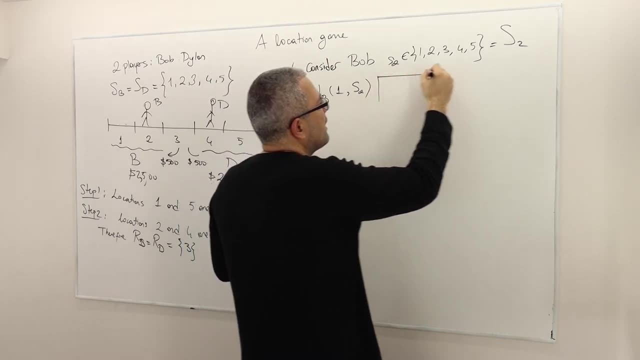 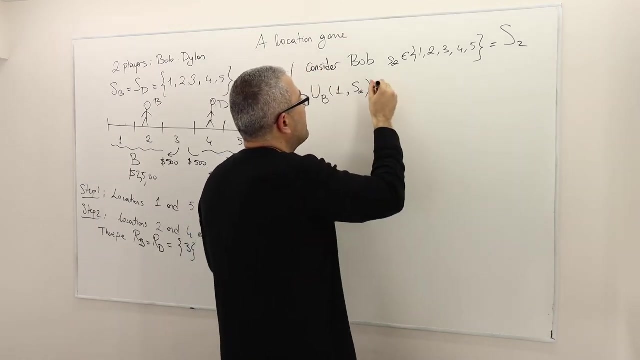 Is to sort of a picture, some sort of a table. all right, So here's what I'm going to do. So I am going to create. Well, this table is going to be too small, Yeah, well, instead of creating a table, let's do this. 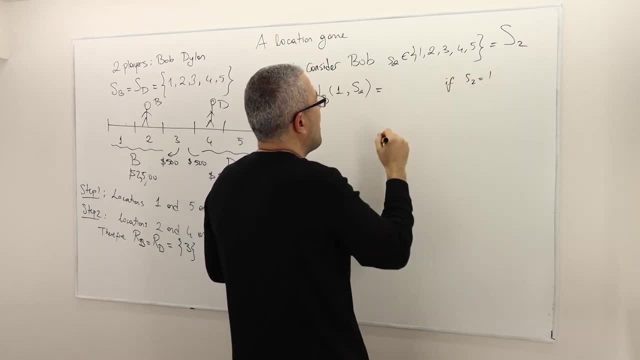 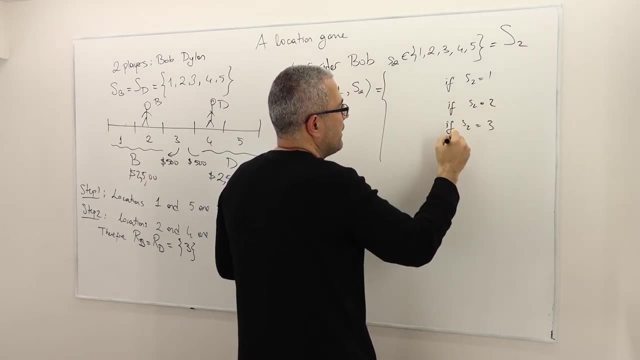 So what is the payoff if S2 is equal to 1?? What is the payoff if S2 is equal to 2?? If S2 is equal to 3?, If S2 is equal to 4, and if S2 is equal to 5,? all right. 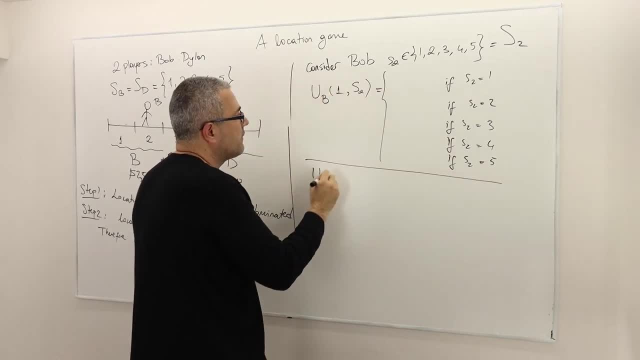 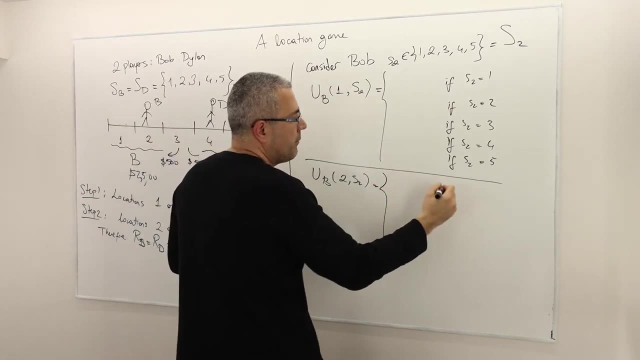 Well then, I am going to, for example, calculate. you know what, if I locate in region 2 instead of 1? What would be the payoff? you know, the profit if S2 is equal to 1,, if S2 is equal to 2,. 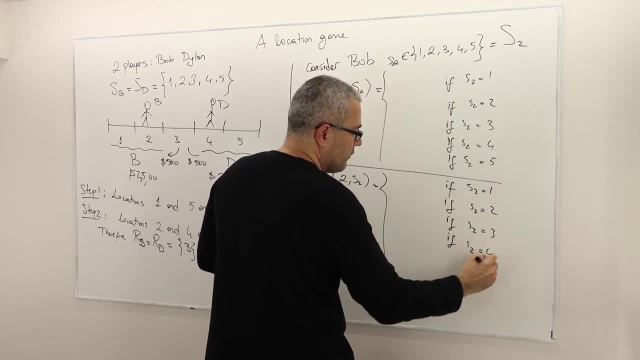 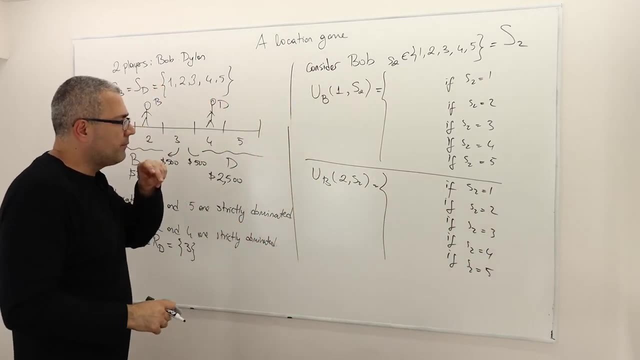 if S2 is equal to 3,, if S2 is equal to 4, if S2 is equal to 5,. all right, I have to do this analysis. Well, can I have? I mean, do I have to do the same thing for U, B, 3, S2?? 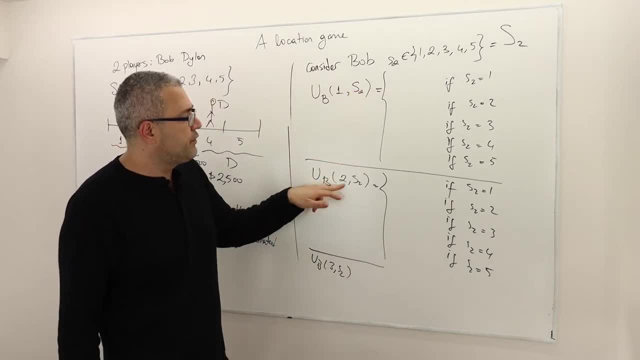 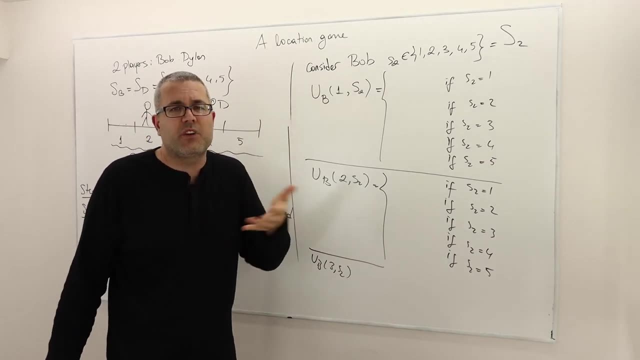 Well, let's first make this comparison: If 2 beats 1, well, that means 1 is strictly dominated. I don't need to find another strategy which dominates 1.. 1 is enough, So therefore I will not need this. 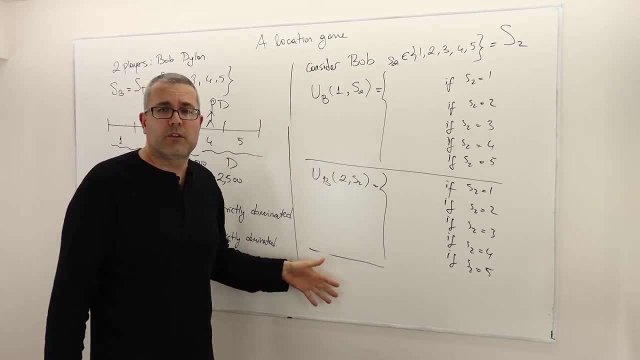 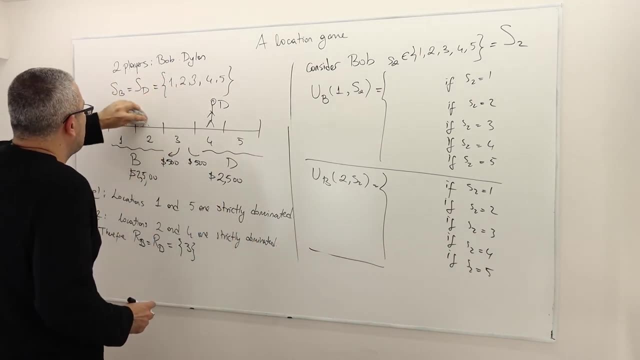 But if 2 does not beat 1,, well then I can go for 3.. If it doesn't, I need to go for 4, etc. All right, So now I'm going to use this table again and again. 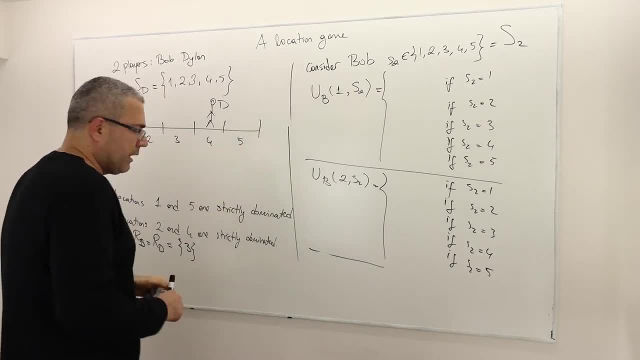 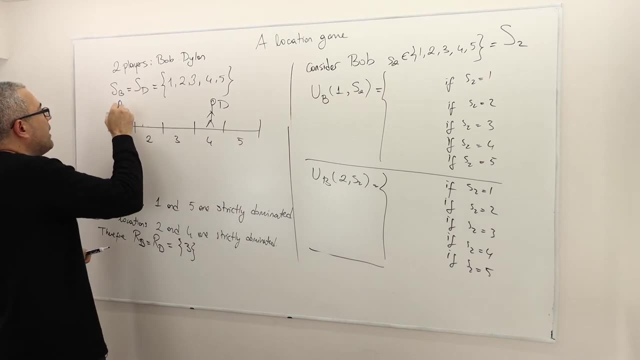 So be careful. What I'm doing is I'm going to put remember Bob into position 1.. So this is Bob and the Dylan, So the Dylan's location will change. Well, first the Dylan will also be here, So both Bob and Dylan are in the same location. 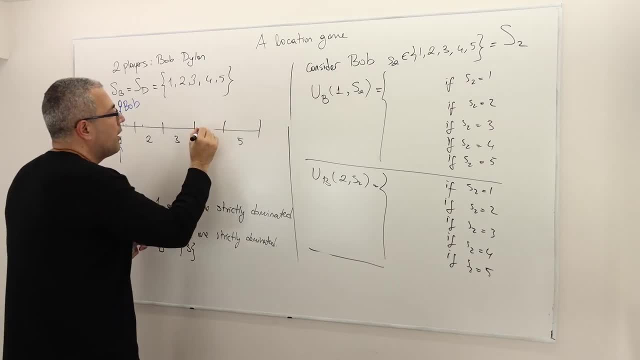 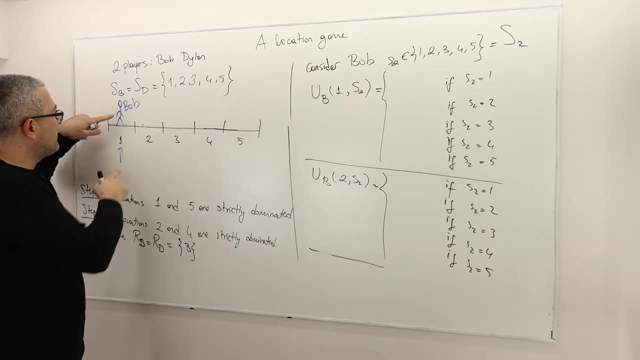 It may take time First, But as you do it more and more you know the calculations are going to be straightforward. You'll see this. So if both guys are sharing the same location, what is going to be? I mean, what regions are they going to serve? 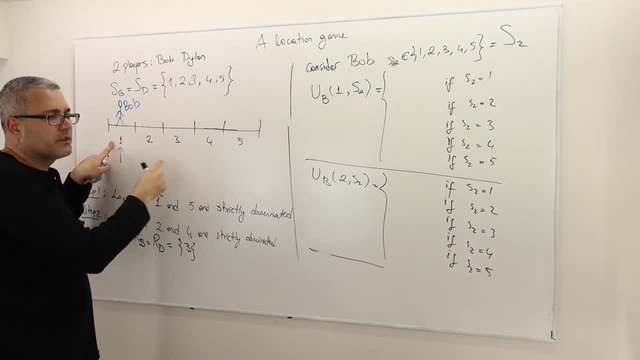 Well, remember, because they are in the same region, all the customers are going to be indifferent between Bob and Dylan. And so remember, in this market there's like 1,000, 2,000, 3,000, 4,000, 5,000.. 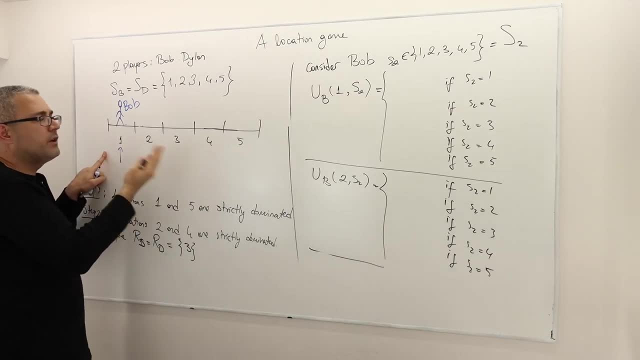 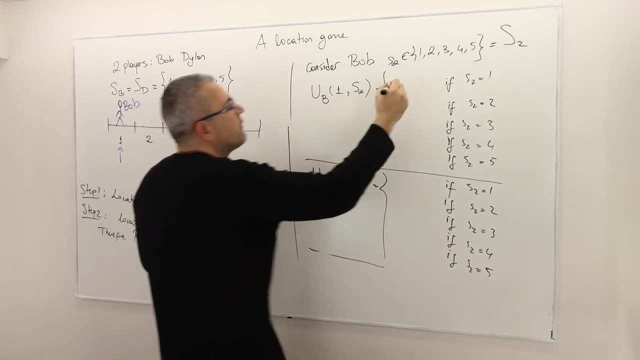 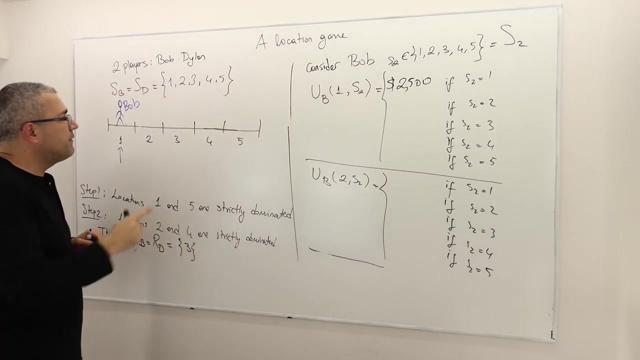 Total of 5,000 net And because the consumers are indifferent between Bob and Dylan, they will equally share, by our assumption. So that means $2,500 is going to be the profit of the Bob. All right If Dylan is located himself in region 1.. 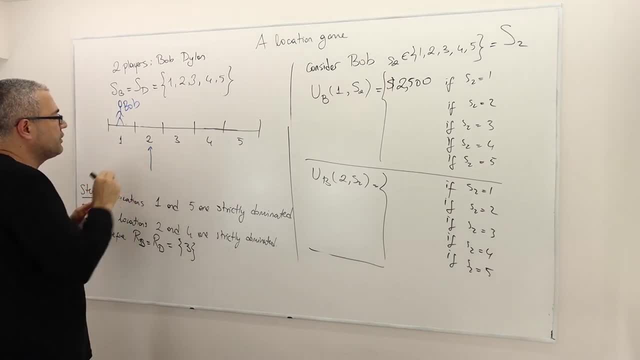 Okay, What if Dylan located himself in region 2?? Well, in this case, all these customers in region 3,, 4,, 5, and 2.. Okay, Are going to select Dylan because you know, in order to go to Bob's restaurant, they all have to walk through the Dylan's restaurant, meaning you know Bob is farther away. 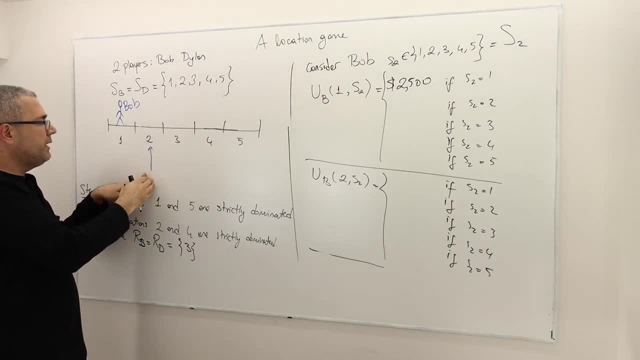 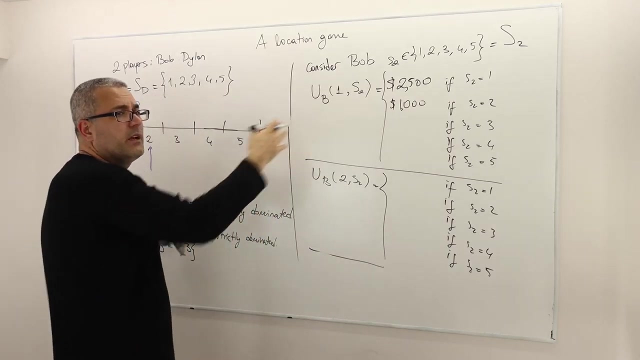 So they're going to go to the closest restaurant, which means Bob will serve only the customers in his own region. All right, So that means his payoff is $1,000.. What is the payoff of Dylan? Who cares? Because I am calculating Bob's payoff. 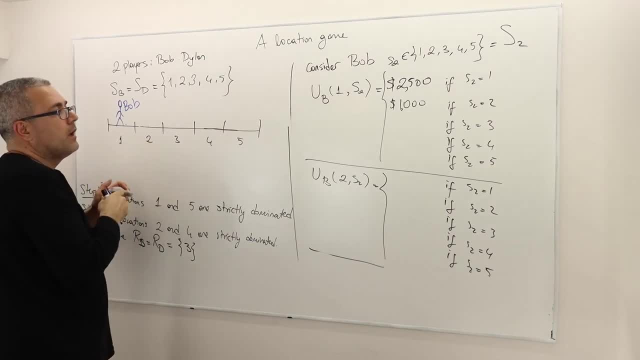 Right, Okay. Well, what if Dylan locates himself in region 3?? Well, this time you know, all these guys are going to go for Dylan. Well, the two guys, half of them will go to Bob, half of them will go to Dylan. 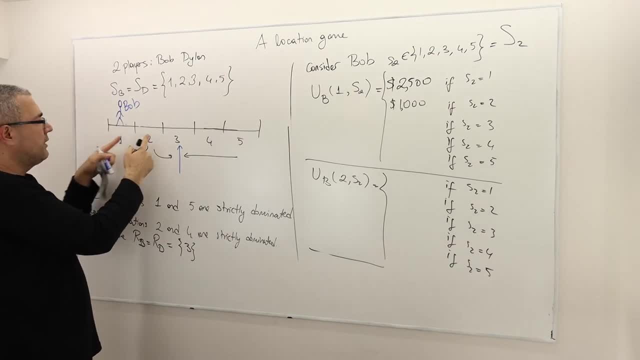 So that means Bob's payoff will be $1,000 plus $500.. So it's $1,500.. So you get the idea All right. Well, what if Dylan? If Dylan locates himself in region 4, you know, all these guys are in region. 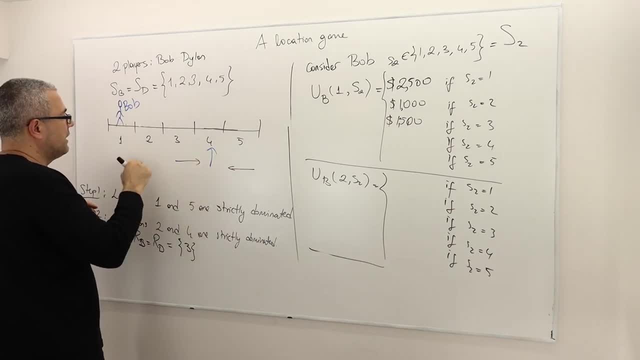 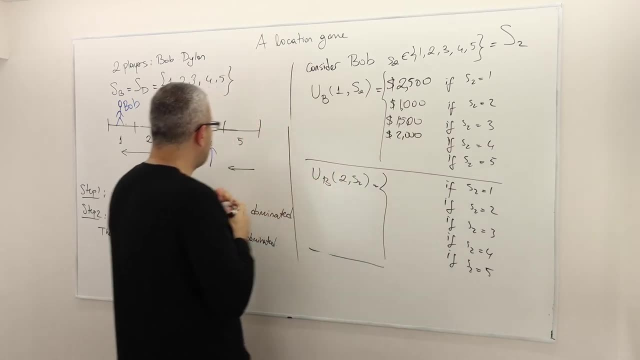 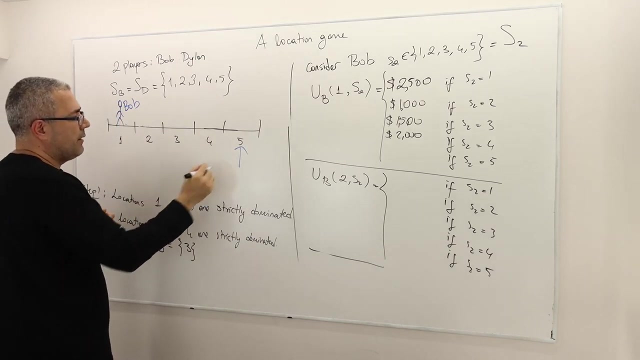 Selects Dylan. Three guys will select Dylan and two and one guys will select Bob. So that means $2,000.. And finally, if Dylan selects himself in region 5, what's going to happen? Well, four guys will select Dylan. 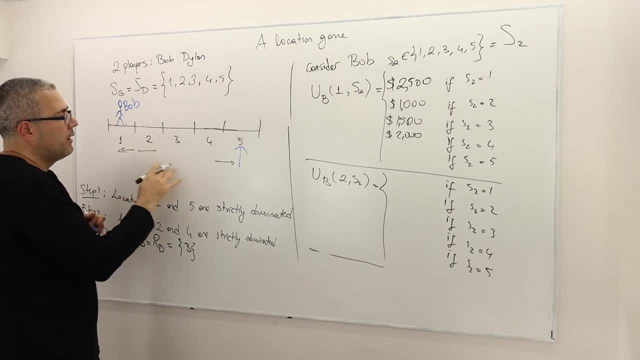 Two guys and one guys will select Bob. The three guys- well, They're going to be completely indifferent, Right? So the half of them will go to Bob, Half of them will go to Dylan. So that means $2,000 plus $500. 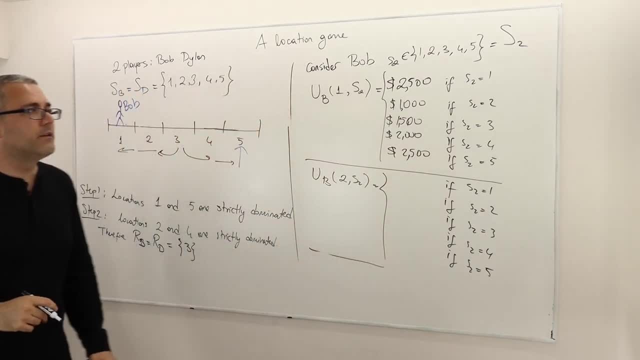 $2,500 is going to be the Bob's payoff. Okay, Now I'm going to calculate those payoffs. So the Bob is not located in region 1, but he is located in region 2.. All right, So this is where Bob is. 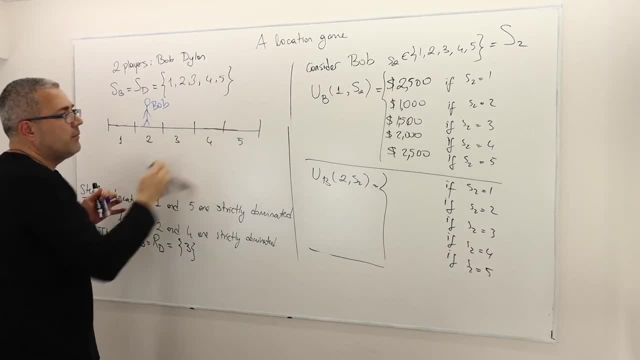 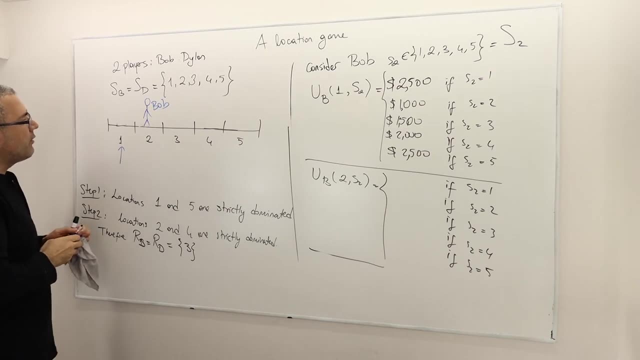 So what I'm going to do? I'm going to do exactly the same thing for, you know, Dylan is in 1,, Dylan is in 2,, 3,, 4, and 5.. Okay, So now, if Dylan is in region 4,, 1,. I'm sorry, I'm going to use the blue color. 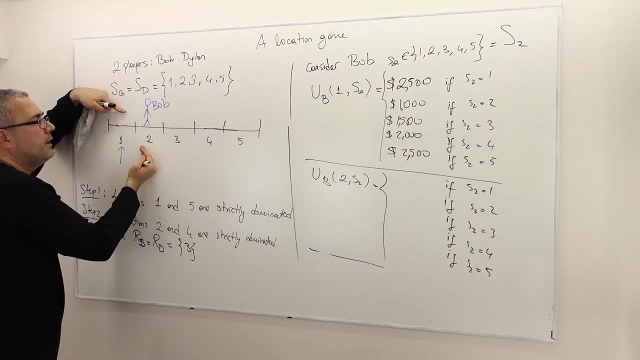 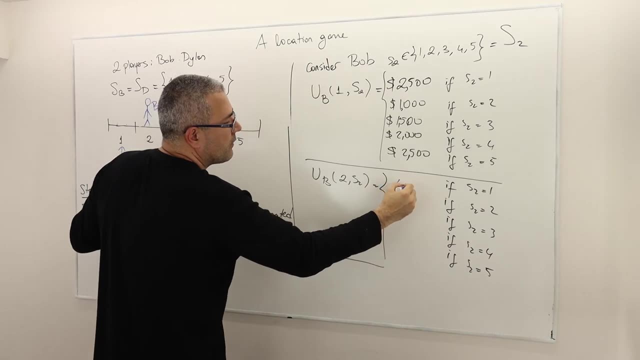 What happens? you know, all these players are going to be selecting Bob's restaurant because he's closer. So that means Bob's payoff will be $4,000.. Clearly higher than $2,500.. Hmm, So you know what? 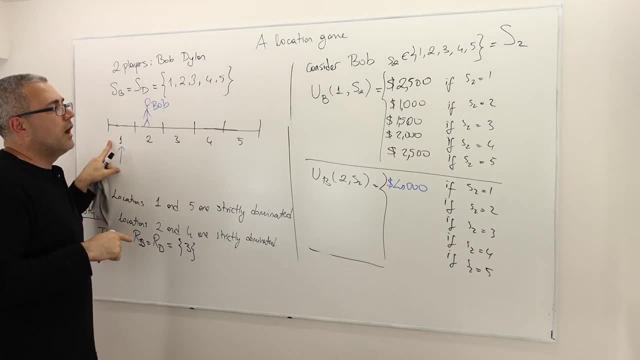 If Dylan selects region 1, for Bob, clearly, region 2 is better than region 1.. Okay, What if Dylan also selects region 2?? Well, because they are in the same region, they're going to share the customers equally. 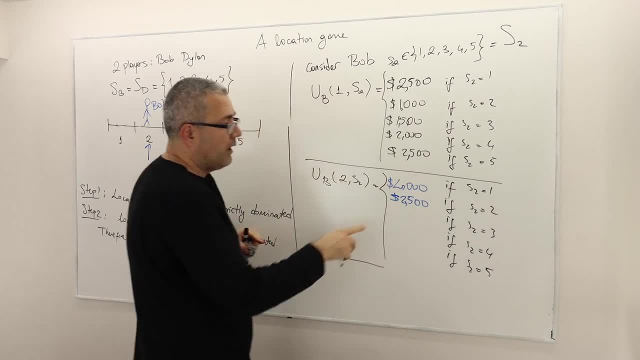 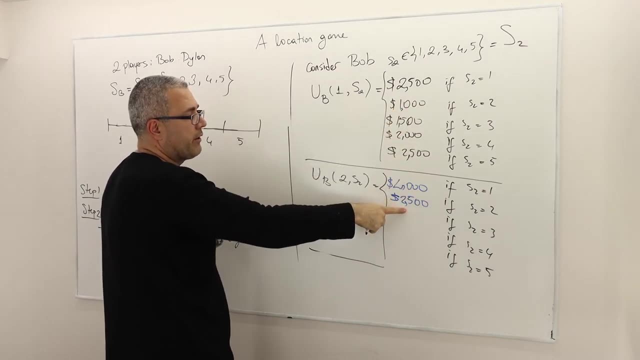 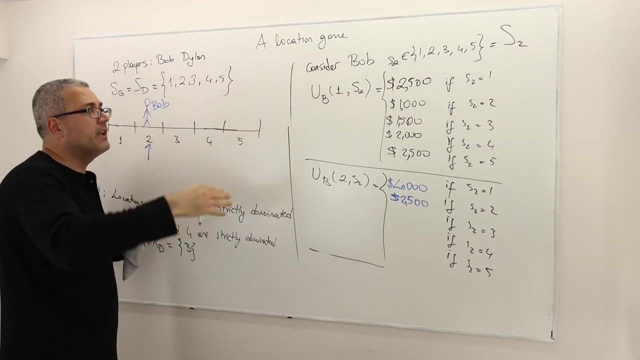 That means $2,500.. Well, again, given that Dylan selects region 2, Bob is actually getting strictly better off If he selects, So if Dylan is in region 2 rather than staying in region 1.. Good, So it seems like 2 is dominating 1.. 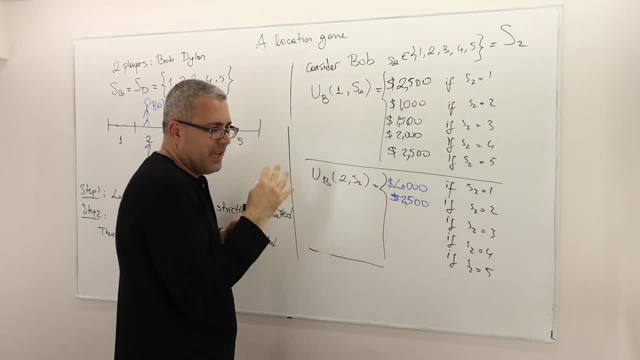 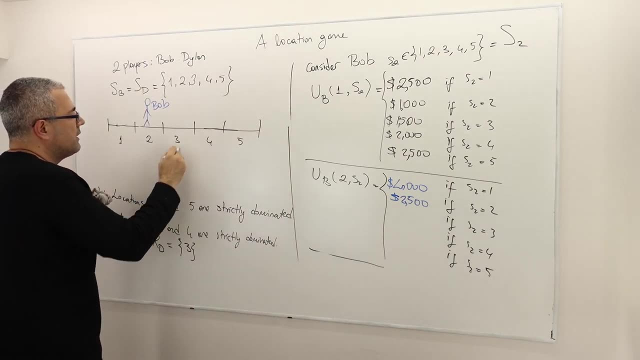 But again, I can't finalize this conclusion. I can't make this conclusion unless I check the other remaining 3 points. All right, What are these 3 points? Dylan is here, Bob is in region 2.. Hmm, So all these guys- region 3,, 4,, 5, goes for Dylan and only 1 in 2 guys goes for Bob. 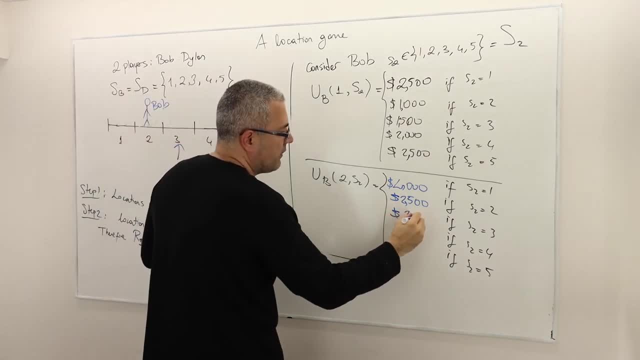 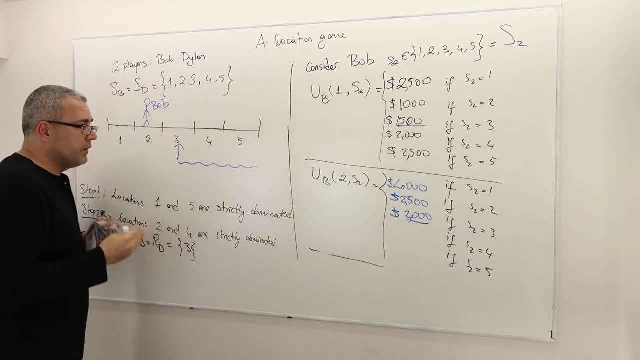 Anyway, the total payoff he will get? Hmm, The total payoff he will get is $2,000, which is higher than $1,500.. Very good, So it seems 2 is really a good strategy in comparison to 1.. 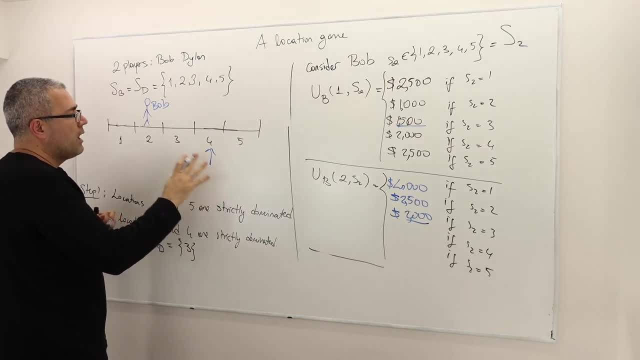 What about Dylan selects region 4?? Well, this time 5 and 4 guys go for Dylan, 3 guys go for. Oh okay, So 3 guys Remember Bob is in region 2, so 3 guys will be indifferent between Bob and Dylan. 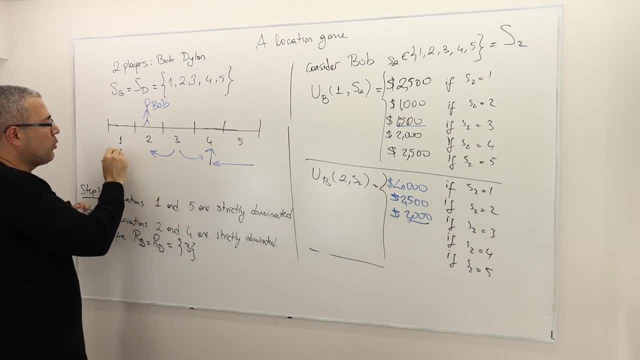 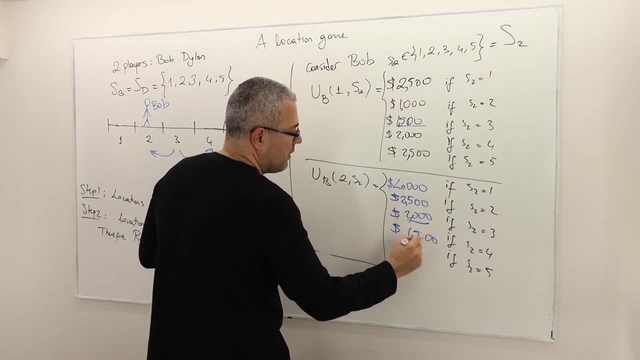 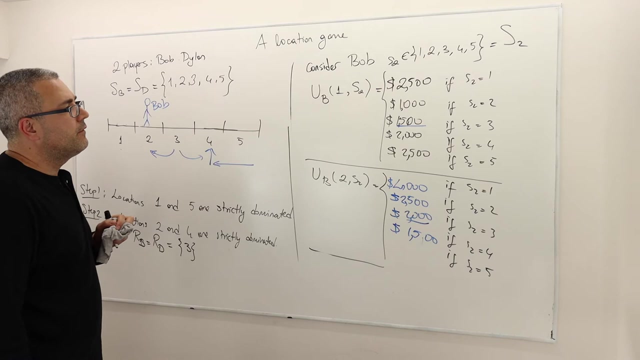 So only Only half of them will go there. So that means $1,000 plus $500,. $1,500 is going to be the payoff of Bob. Hmm, All right, Very good, That's no good news. 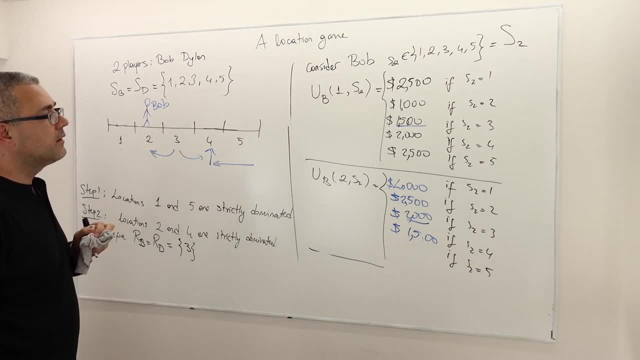 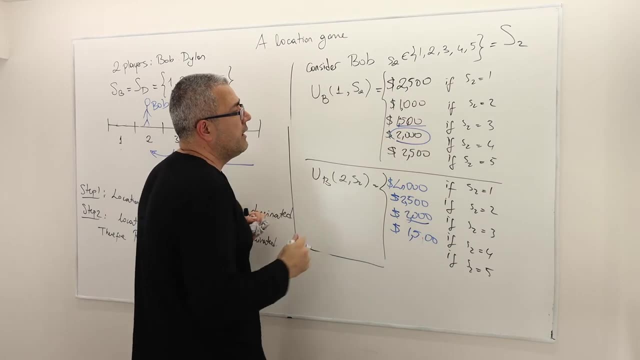 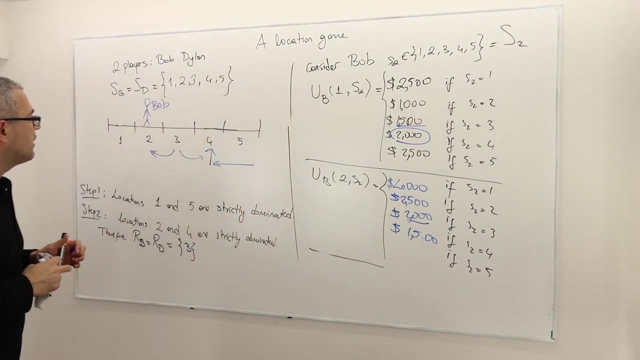 Right, Yeah, That's. Why is that so Well, because remember, locating yourself was giving $2,000, but locating yourself to 2 is giving you $1,500.. Oh, I'm sorry, That's my bad. 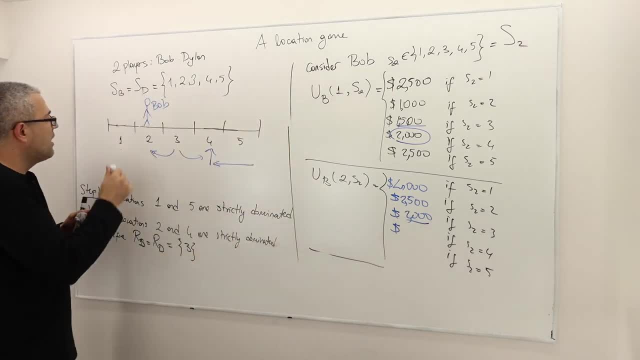 So you have to be very careful. This is not $1,500. It's more than that. Why People in region 1 selects Bob, People in region 2 selects Bob. Half of the people in region 3 selects Bob. 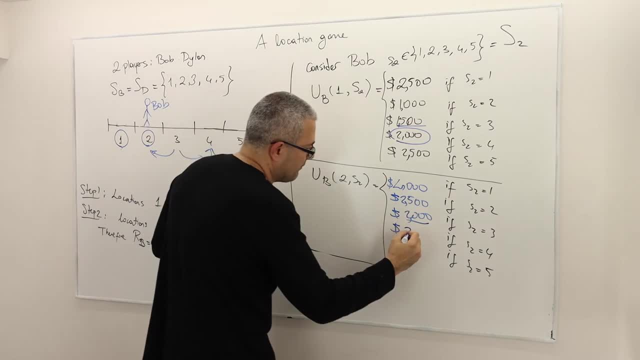 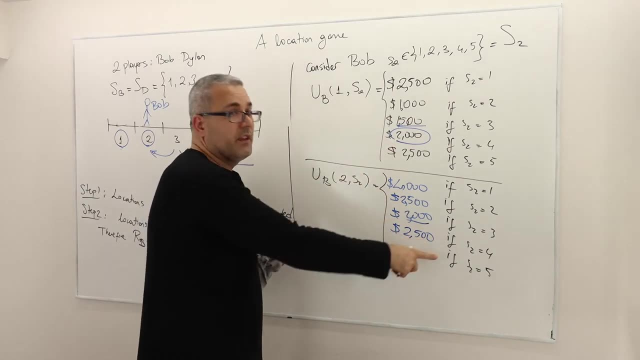 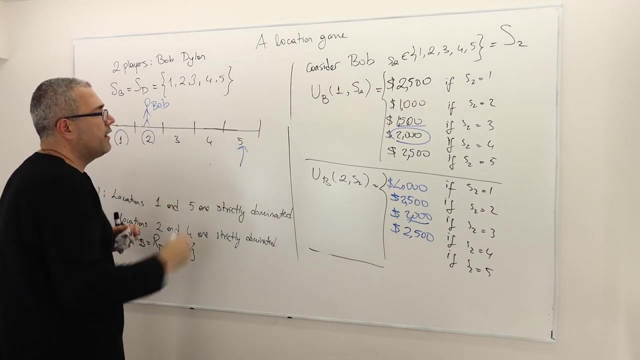 That means it's $2,500.. Nope, There you go. Be careful. So, okay, 2 is better than 1, also in this case. And then one final case: What if Dylan selects region 5?? All right, 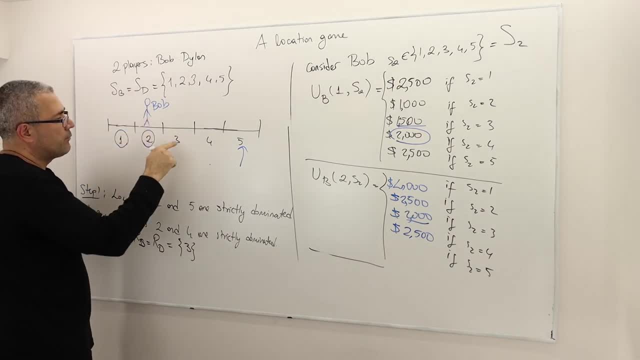 In region 1, selects Bob. Region 2, selects Bob. Region 3,. well, it's like two steps to Dylan but only one step to Bob. So they're going to choose Bob And Player in 4, well, it's two steps to Bob, but one step to Dylan. 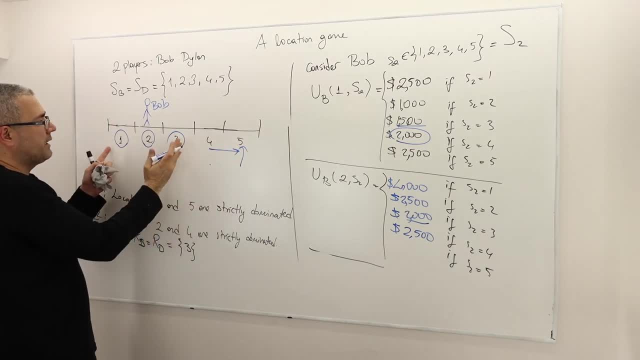 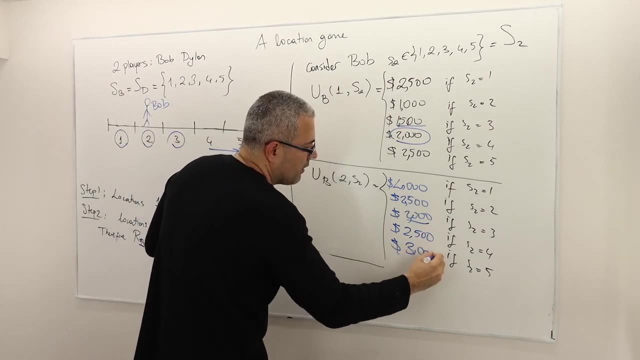 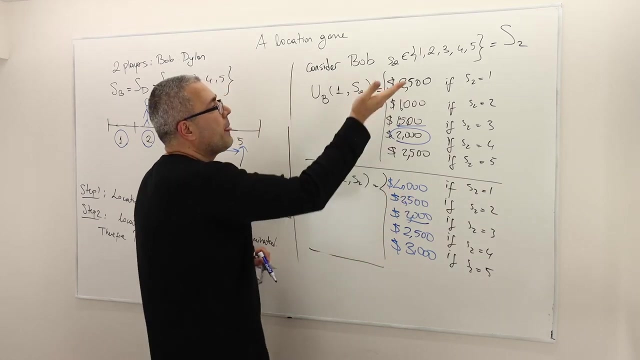 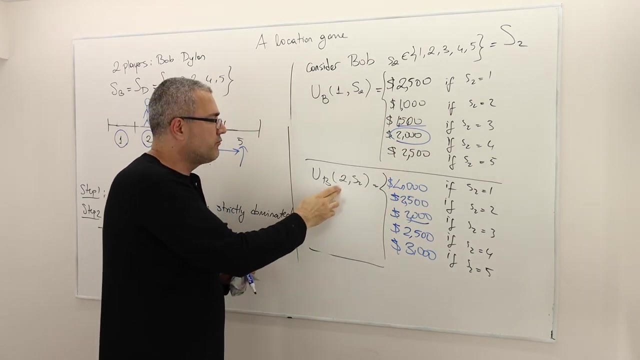 So they're going to go for Dylan. So that means Bob is going to get Will going to serve these three regions. That means $3,000, which is higher than $2,500. So you know what, Whatever Dylan does, Bob's payoff will be always strictly higher if he locates himself in region 2,. 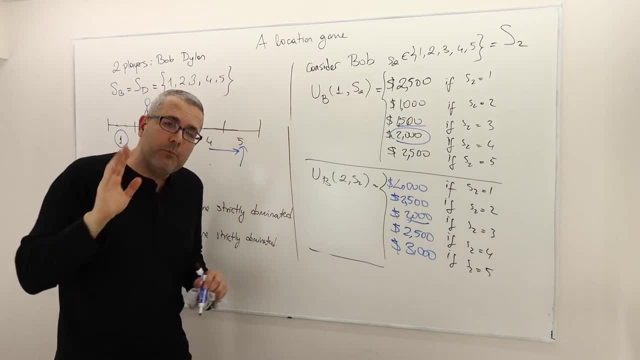 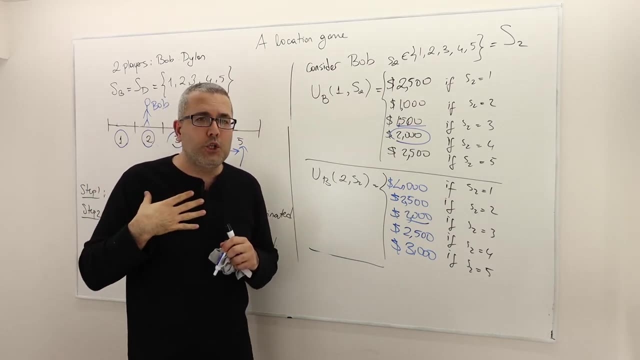 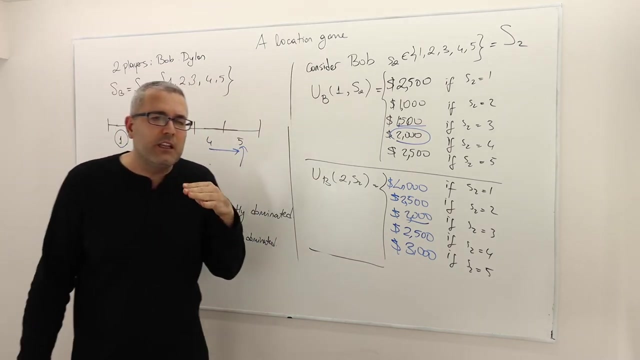 rather than region 1.. So be, I mean be careful Here. I am not finding the best strategy for Bob or Dylan. What I'm showing is that playing strategy 1 or locating your restaurant in region 1 is definitely worse strategy, regardless of your opponent's behavior. 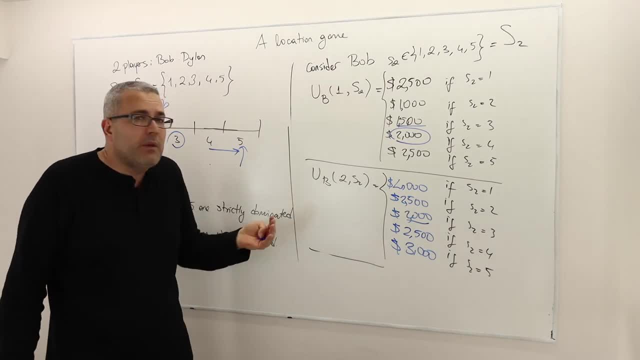 than locating yourself in region 2.. Maybe locating yourself in region 3 is better than locating yourself in region 2.. I don't know. At this point I don't care. All I want to know is that locating yourself in region 1 is a strictly dominated strategy. 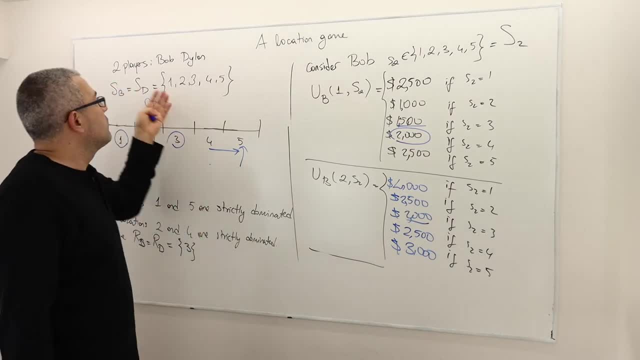 So, therefore, a rational Bob, or Well, by the way, I mean, everything is symmetric for Bob and Dylan, right? The payoffs are symmetric, etc. So if these arguments are true for Bob, they are also true for Dylan. 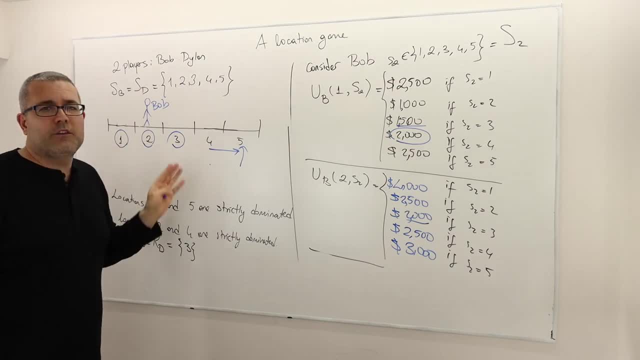 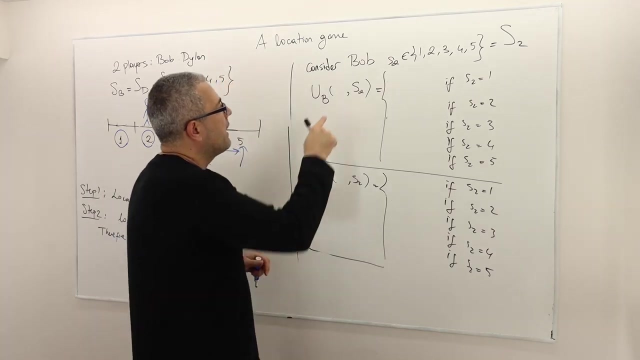 So that means playing strategy 1 is out of the picture. Bob shouldn't be playing, locating his store in 1, and Dylan, symmetrically, shouldn't be locating himself in region 1.. All right, So what I'm doing now is: let's suppose Bob locates himself in region 5. 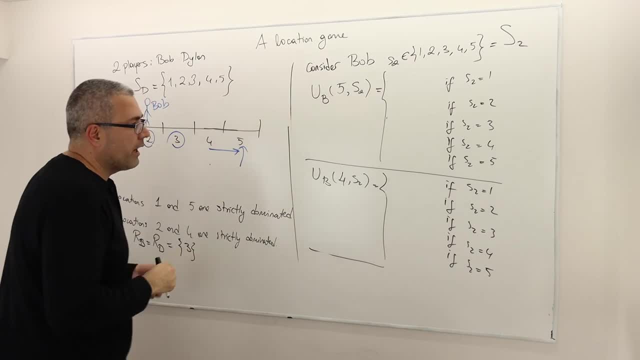 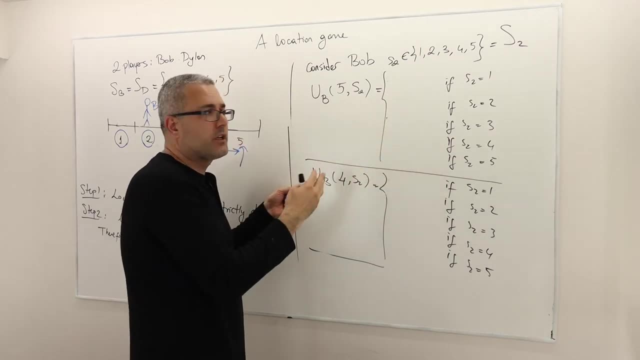 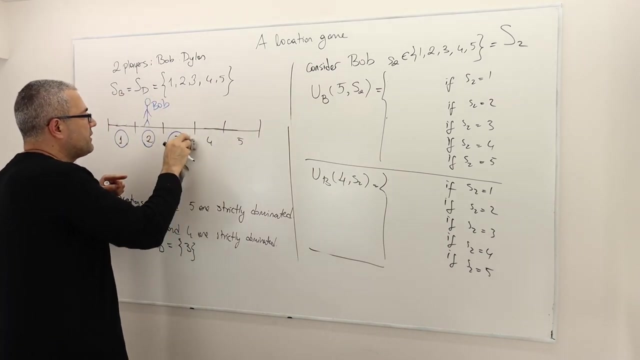 versus. he locates himself in region 4, all right, And I am again going to hopefully show that the payoffs here are going to be better than the payoffs here. So locating in the extreme, You know, the other extreme or the other opposite end of this beach. 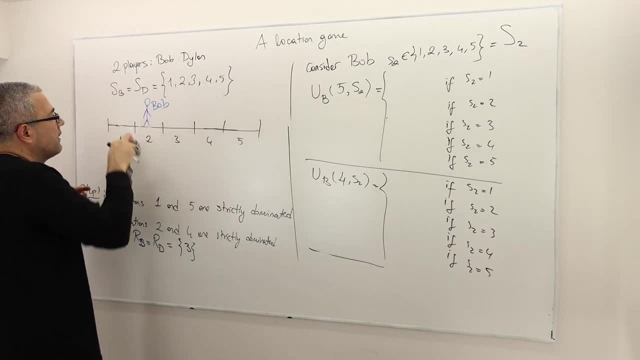 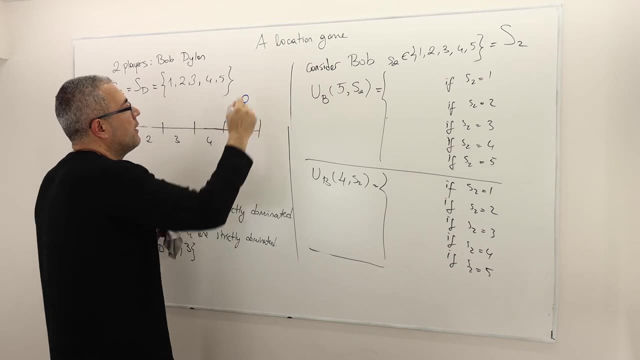 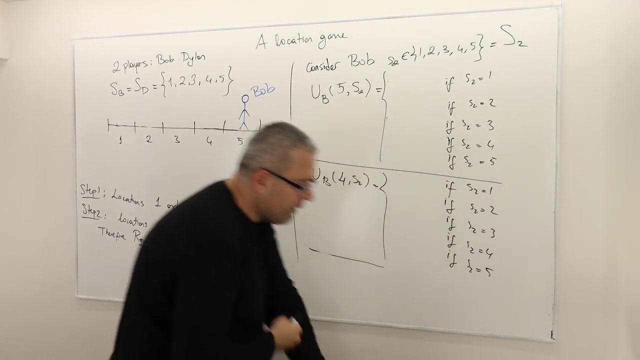 is not profitable for Bob or Dylan. So let's put Bob here. So here is Bob. All right, So he's in, located in region 5.. So now let's calculate. So I'm going to be a bit faster. 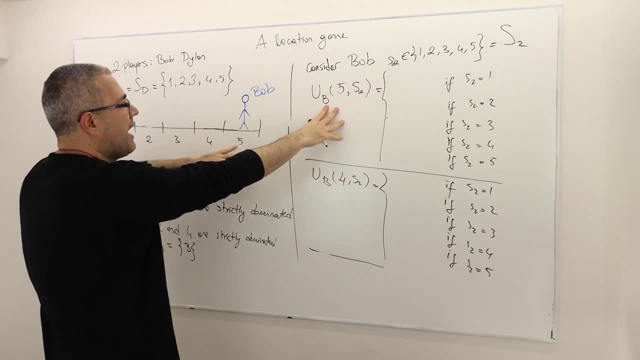 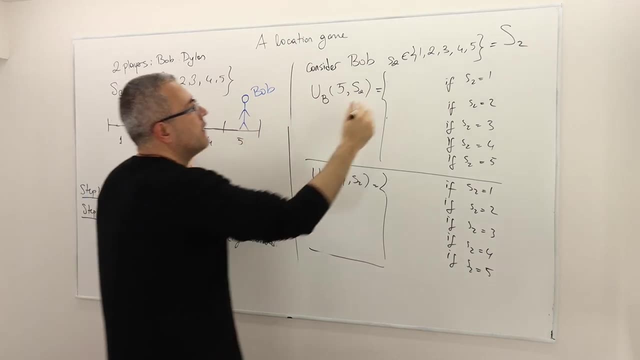 So if Bob is in located in region 5 and Dylan is in in region 1, what happens is that they're going to split the market equally, So it's going to be $2,500.. However, if Dylan is located here, 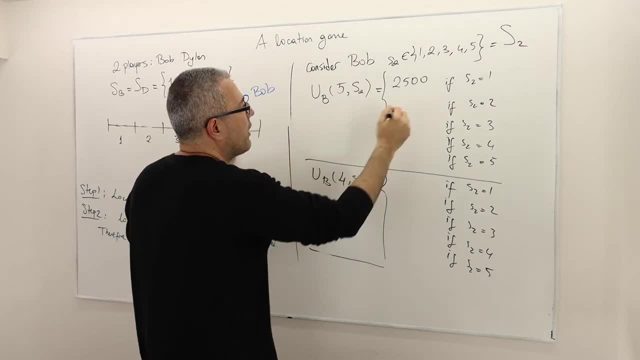 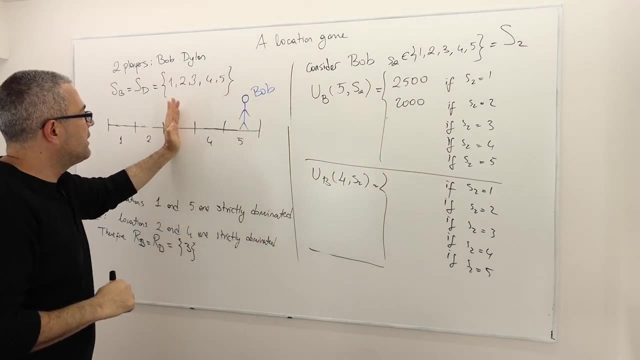 what's going to happen is only two markets, 4 and 5 will be coming to Bob's store. It's going to be $2,000.. However, if Dylan is located here, what's going to happen? they're going to split the region 4.. 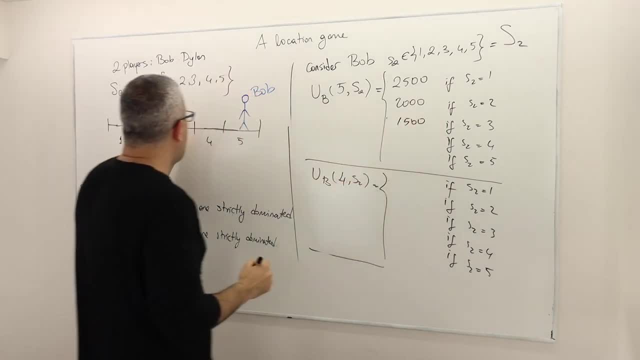 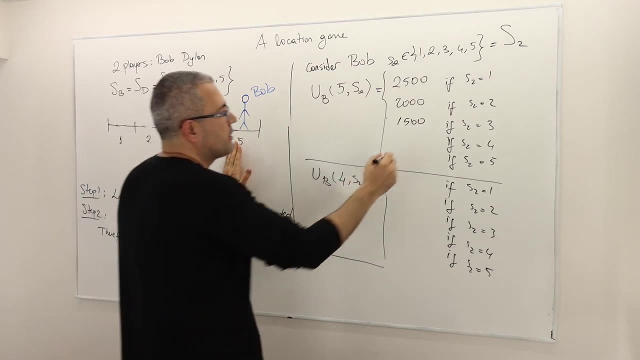 So it's going to be $1,500.. And if Dylan is located here and Bob is located in region 4, what's going to happen? Dylan is going to get everything here, Bob is going to get just region 5.. 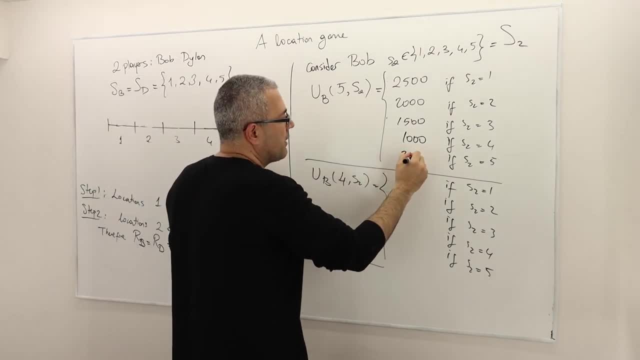 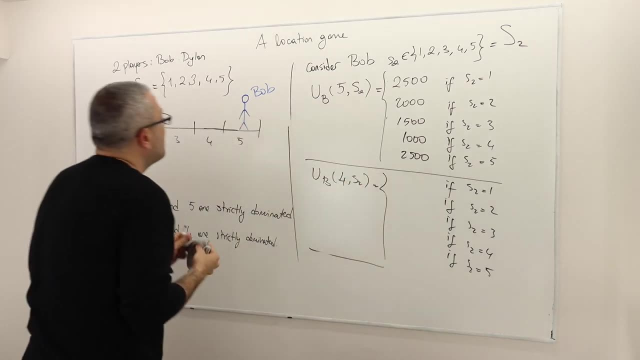 And if they both located in region 5, they're going to split the market equally. So these are going to be the payoffs. Well, now let's look at the environment, where Bob initially actually locates himself in region Oops. 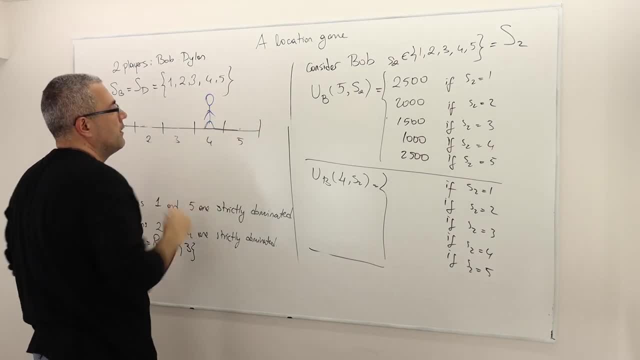 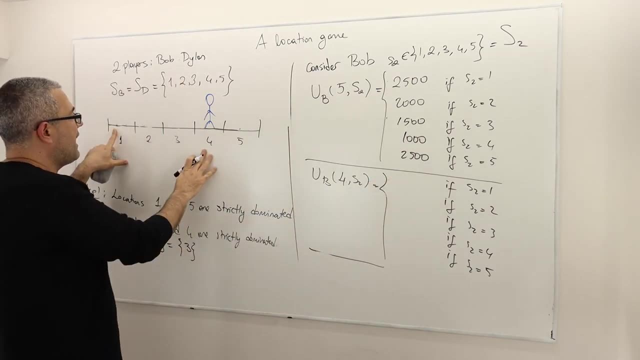 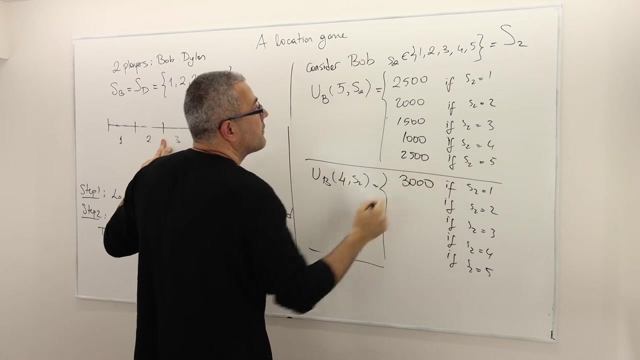 Sorry, In region 4.. All right, Okay. So if Dylan is located in region 1, what's going to happen? the Bob is going to serve everybody in region 3,, 4, and 5.. So payoff will be $3,000. 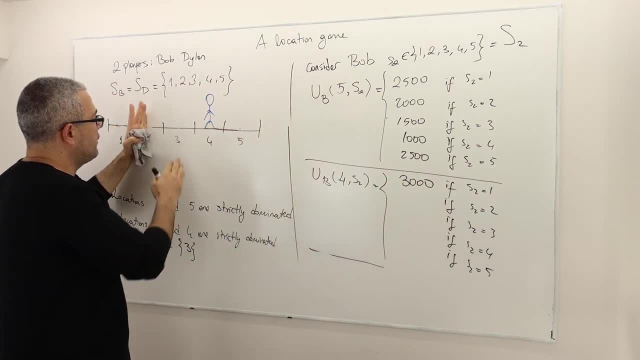 If, however, Dylan is located 2,, what's going to happen? They're going to split 3.. And so it's going to be $2,500.. If Dylan is located here, it's going to be 4 and 5.. 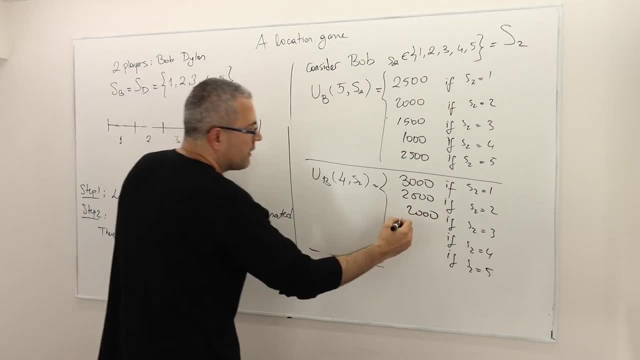 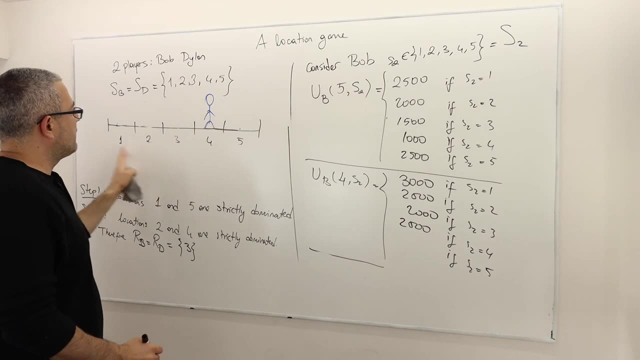 So $2,000.. If it's located 4, they're going to split equally. If it is located 5, what's going to happen? The Bob is going to get all these guys. So it's going to be $4,000.. 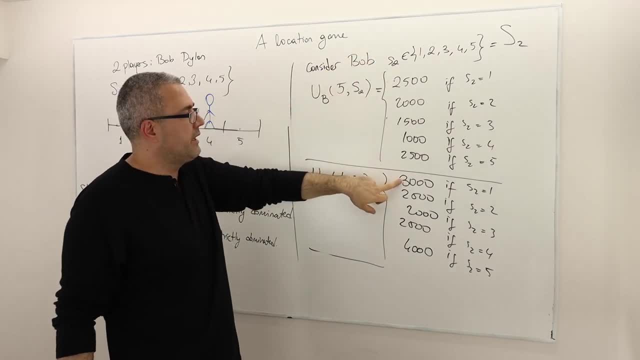 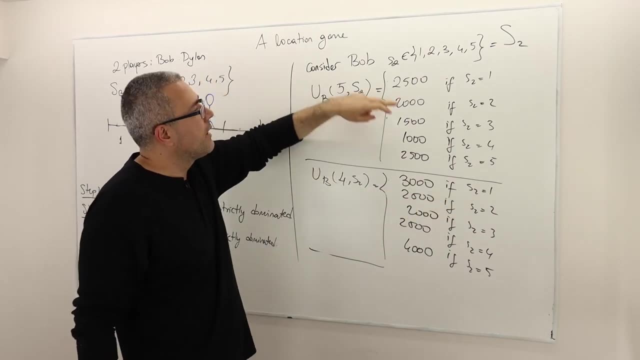 So $2,500 versus $3,000.. So 4 is a better strategy than 5,, at least when the second guy plays 1.. $2,000 versus $2,500.. So 4 is still better. 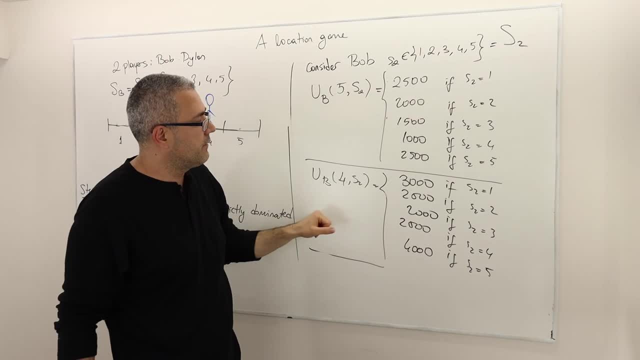 $1,500 versus $2,000.. $1,000 versus $2,500.. $2,500 versus $4,000.. So you see, whatever Dylan does, Bob's strategy of locating himself towards the center. that's the idea. 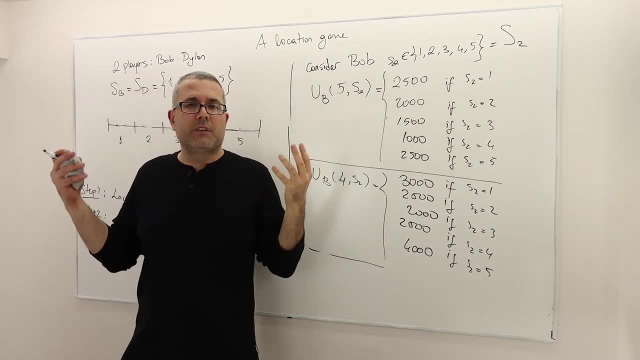 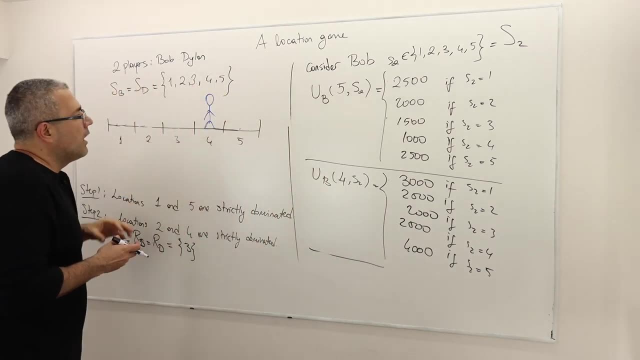 I mean there's nothing special about the extremes. It's sort of the center is the- I don't know the center of gravity kind of force. So as Bob gets closer to the center he actually serves more of both sides of the market. 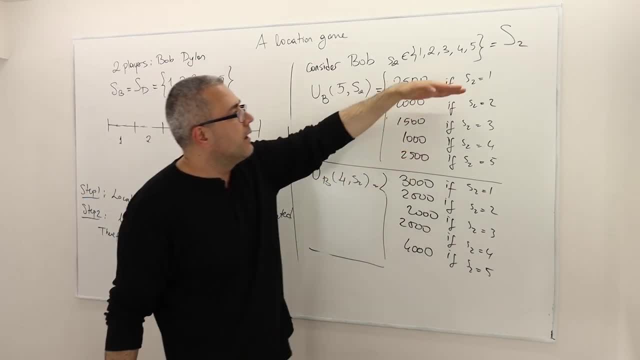 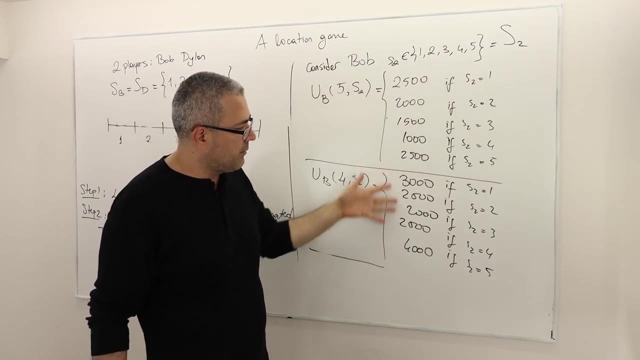 All right, And so obviously the Dylan's strategy is going to change his total payoff. Sometimes it's going to be less, Sometimes it's going to be more- More than $2,000 or less than $3,000.. But the thing, the idea is. 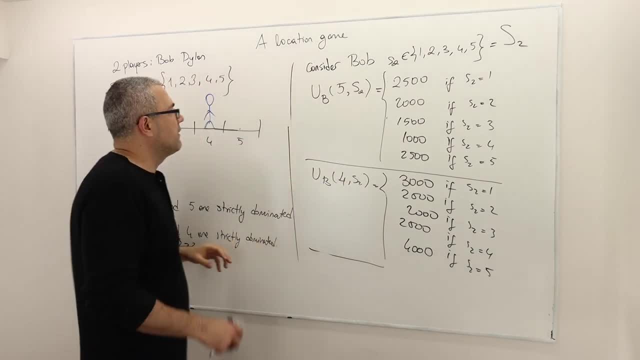 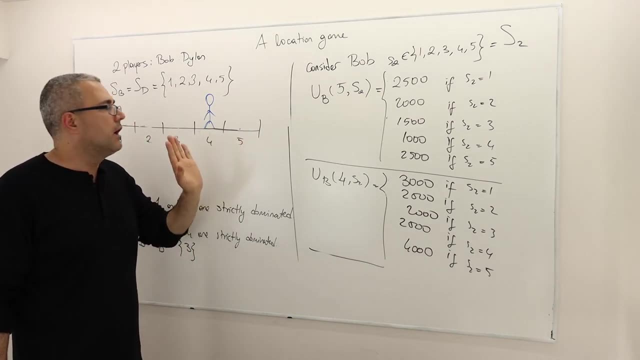 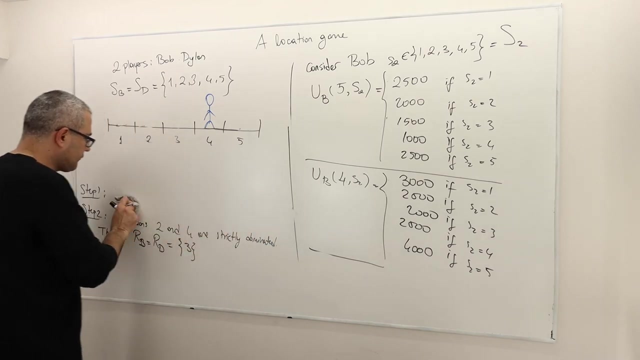 playing 4 is definitely a better strategy than playing 5.. So again, rational Bob and rational Dylan should never look at, should never locate their stores in region 5.. So what does that mean? That means after step 1,: 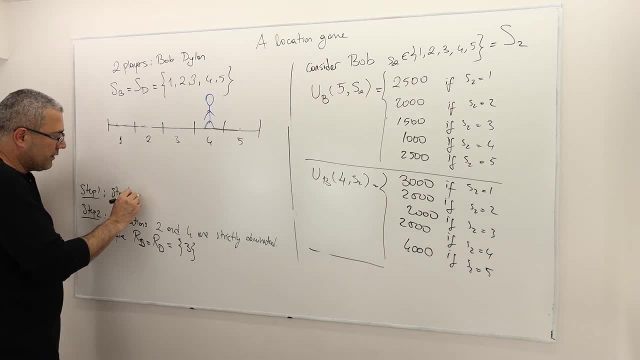 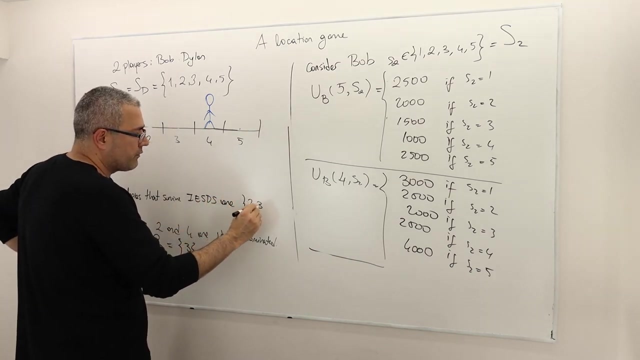 the strategies: strategies that survive, iterated elimination of strictly dominated strategies, IESDS- iterated elimination of strictly dominated strategies- are 2, 3, and 4.. But be careful, That doesn't mean that region 5 and 1 out of question. 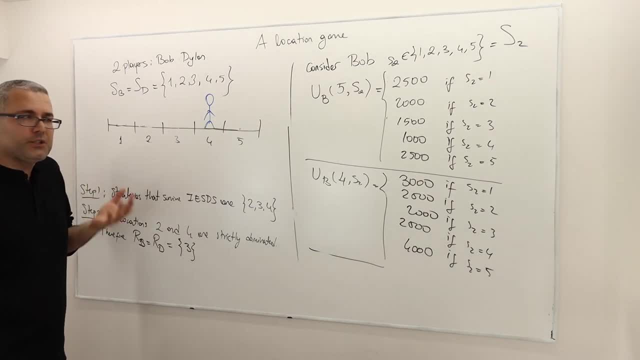 It's just well. these people, these customers, still need to be served. But the thing is, you know, these strategies are no longer available for Bob and Dylan because they are irrational strategies. So what does that mean? That means in the second step. 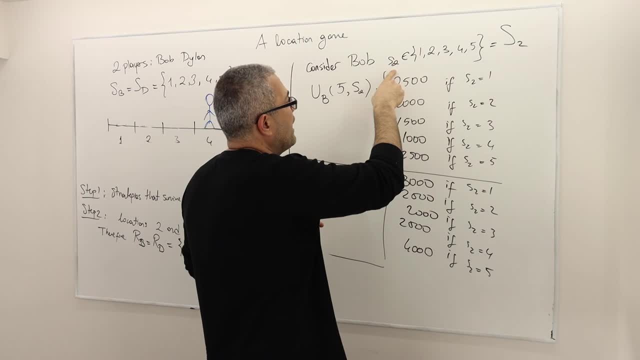 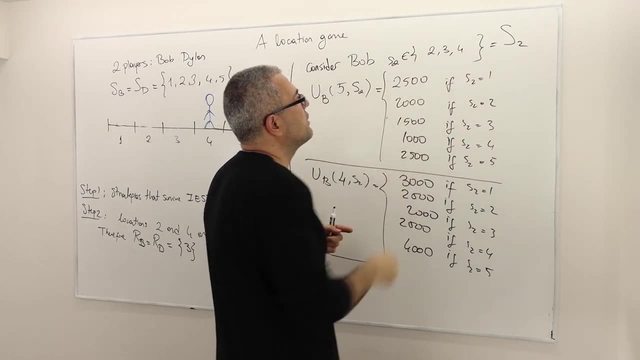 my analysis is going to be the following: Look, S2 is no longer coming from 1,, 2,, 3,, 4, 5, because I know 1 is irrational, 5 is also irrational, So therefore, S2 should be coming from 2,, 3, 4.. 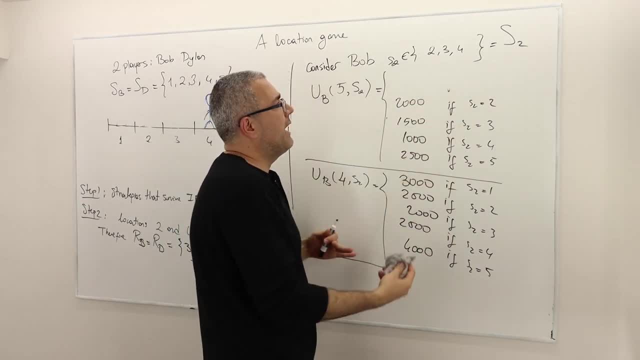 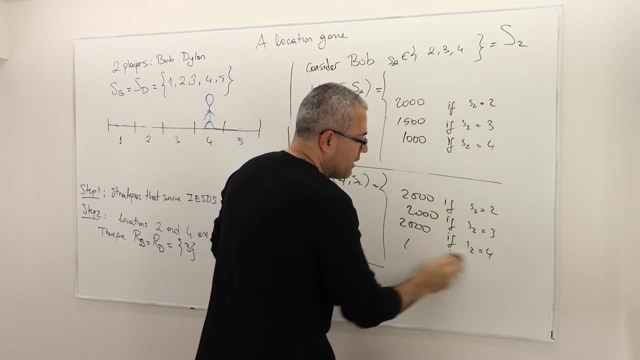 That means, when I make comparison now, I'm not going to, I'm going to ignore S2 equal 1 and S2 equal 5, and also this. So what I need to do now is to make comparison between these three, with these three. 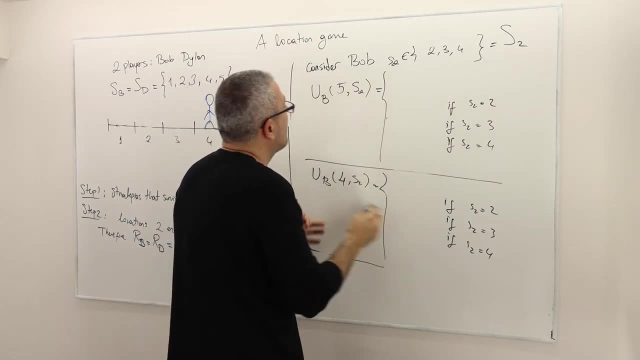 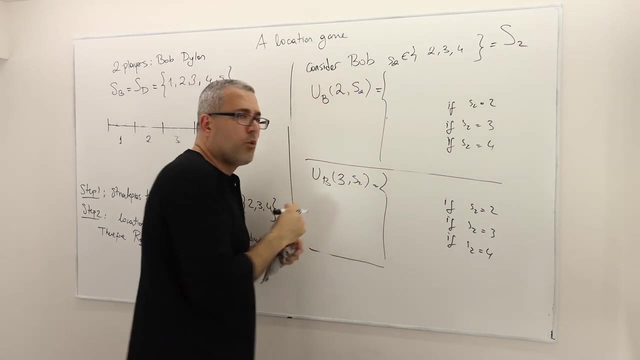 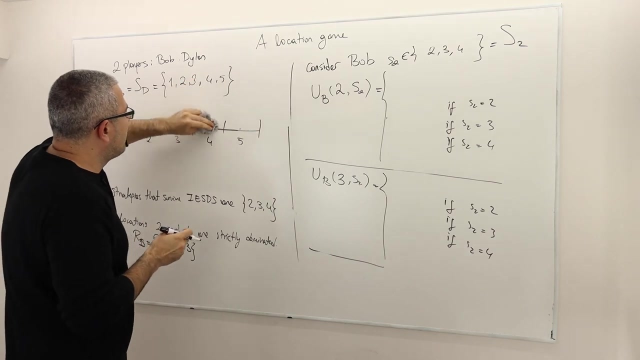 All right, So let's do it. For example, the Bob locates himself in region 2 versus region 3. Sort of more central location, All right, So okay, So the Bob locates himself. I'm going to put Bob on black color now. 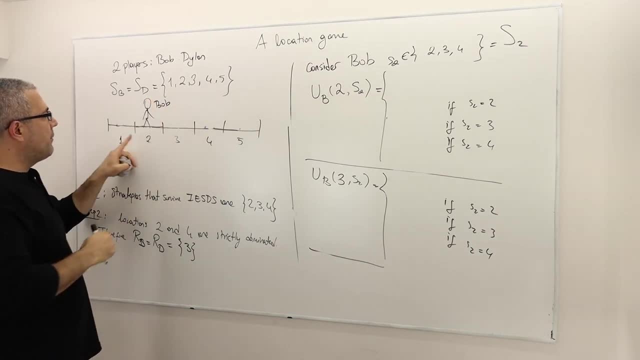 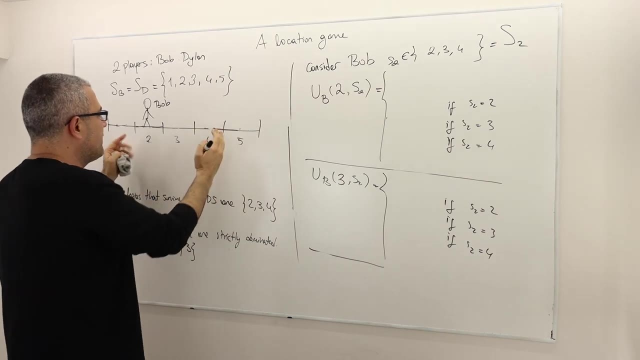 for no reason. So this is Bob. So when Bob is in region 2, well, if Dylan is also in region 2, they're going to share the entire market. Remember, the market is not just 2,, 3,, 4.. 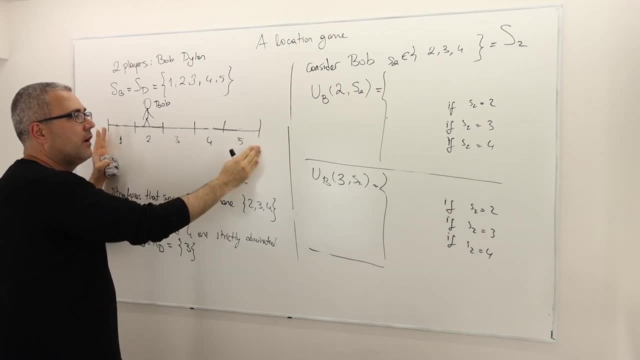 The market is all the customers from 1 to 5.. Okay, So therefore it's going to be 2,500.. However, if Dylan locates himself in 3,, well, that means only 1 in 2 customers will select Bob. 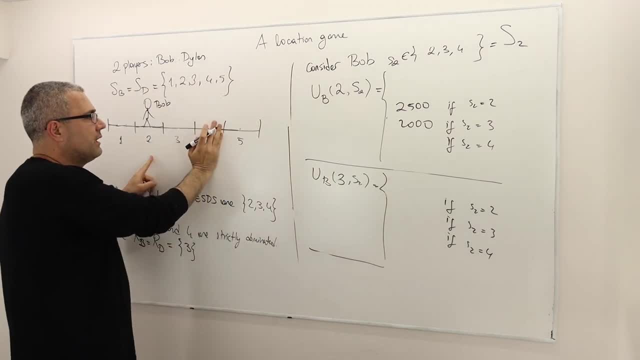 So it's going to be 2,000.. And if he, if Dylan, locates himself in 4,, well then that means they're going to share the customers in region 3.. So it means 2,500. 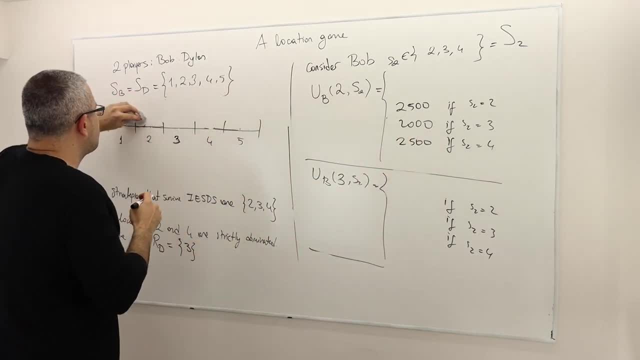 Well, what if Bob locates himself in region 3 instead? Well, this time, if this is the Dylan's location, well, all these guys are going to Dylan, All these guys are going to Bob, So it's going to be 3,000.. 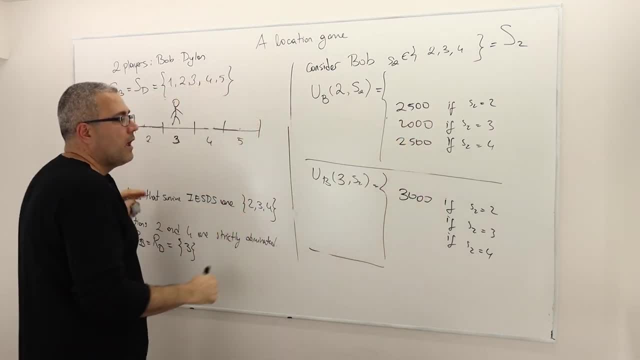 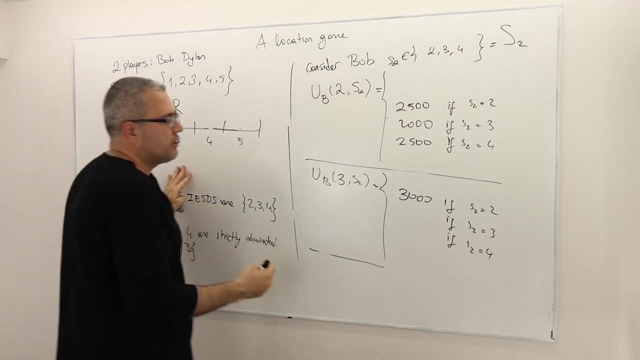 Higher than 2,500.. Good Well, what if Bob also locates himself- I'm sorry, Dylan also locates himself in region 3?? They're going to be sharing market. They're going to be sharing market equally. So 2,500 went, better than 2,000.